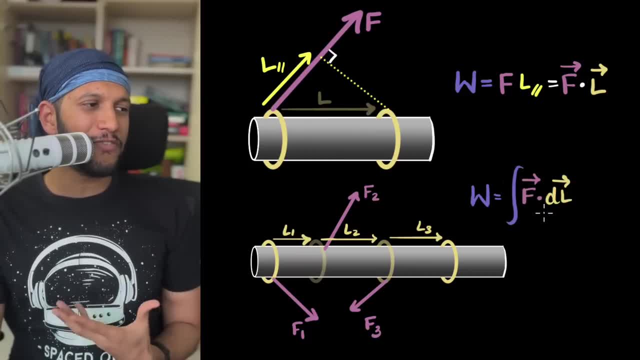 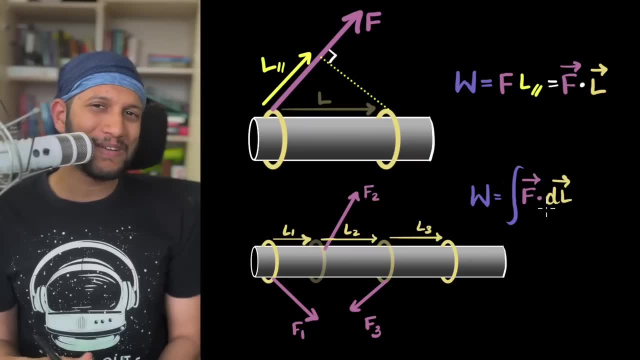 you end up getting an integral. So that's the general form of calculating work done. Wait a second, Feynman, are we going to do integrals in this video? He says, no, don't worry about it, We don't need to do any integrals. Cool, All right With that. basics. 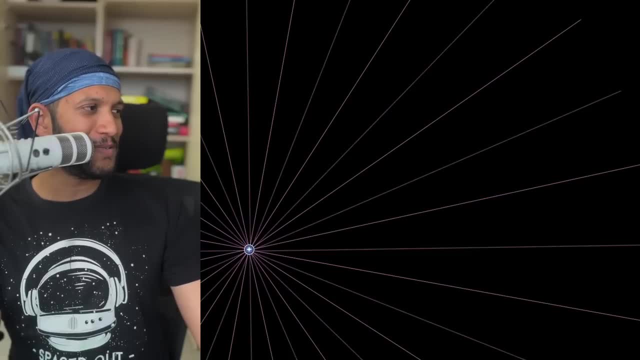 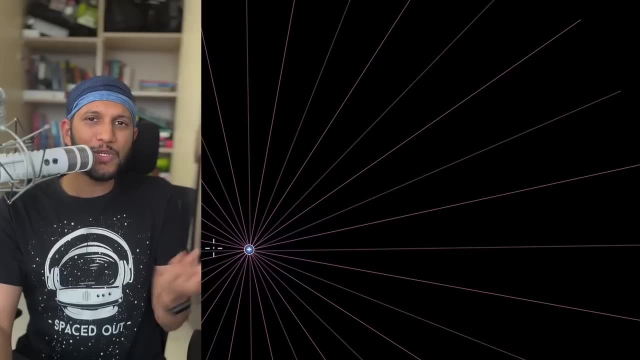 where do we start? Well, Feynman says: consider a point charge. Now, a point charge gives out a radially symmetric electric field, right? Well, guess what? That's what you write in an equation form and you'll get your Maxwell third equation. I'm like what? How do I write the fact that 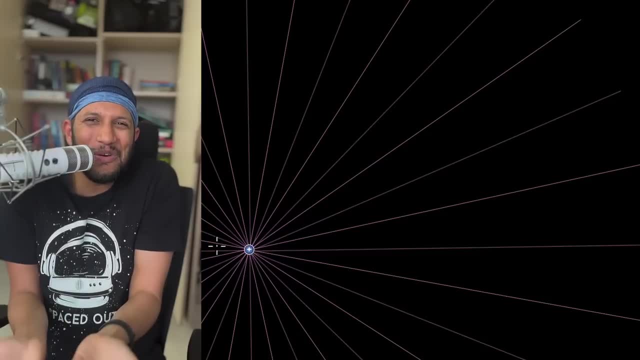 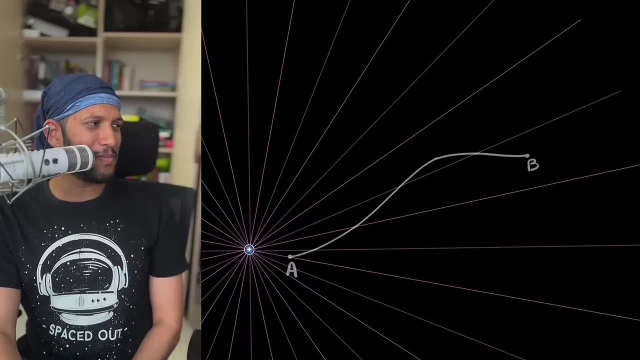 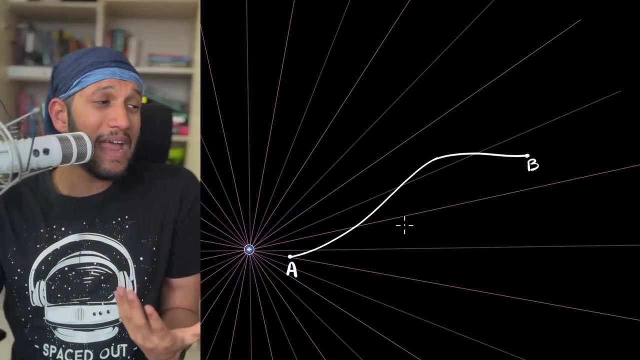 the field is radially symmetric in an equation format. How do I write that? Here's how says Feynman: Well, take a unit charge, move it from some point A to point B and think about the work done. This work done will not depend on the path taken, Because the 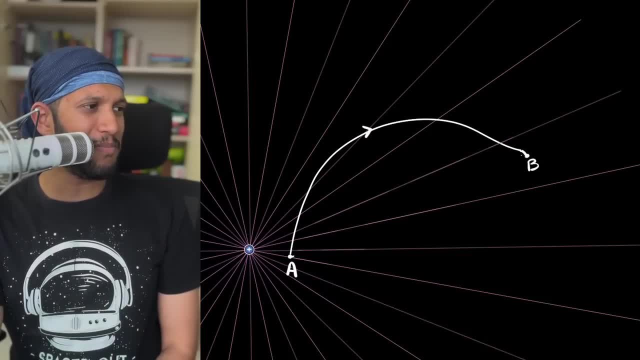 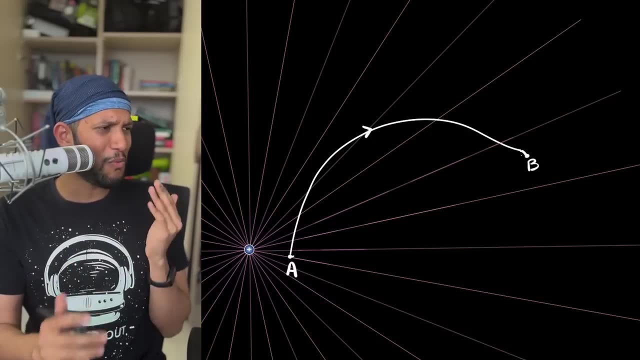 field is radially symmetric, whether you take this path or this path, the value of the work done would be the same, regardless of what path you take. Wait a second, wait a second, wait a second. I'm not sure Why. Why, if the field is radially symmetric, the work done does not depend on the 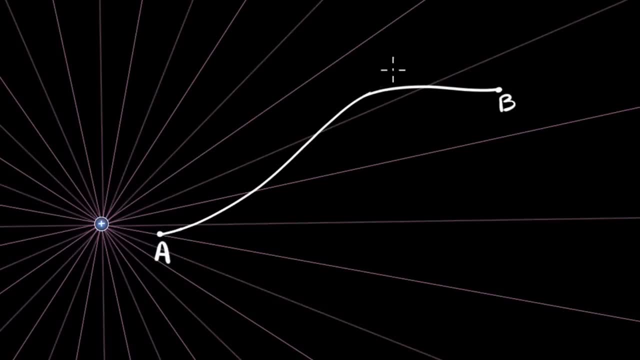 path. Here's why, says Feynman, If you consider this particular work done along this path, well, the forces are changing Right, So we need to divide this into tiny, tiny sections. Let's consider a tiny section over here. 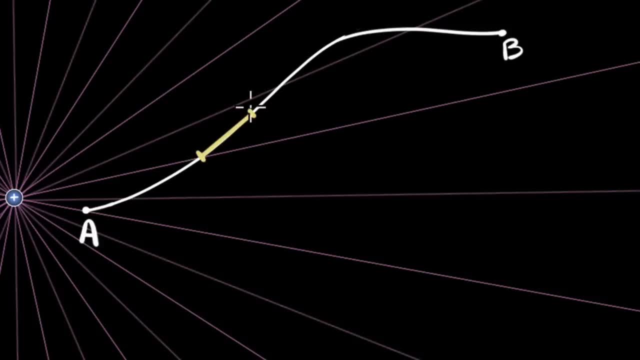 and think about the work done in moving that unit charge from here to here. Well, at that particular location, the force will be along the field line, so the force will be this way. And so to calculate the work done, we take the component of the. 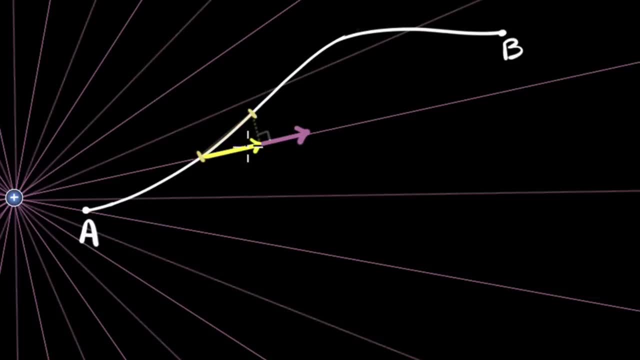 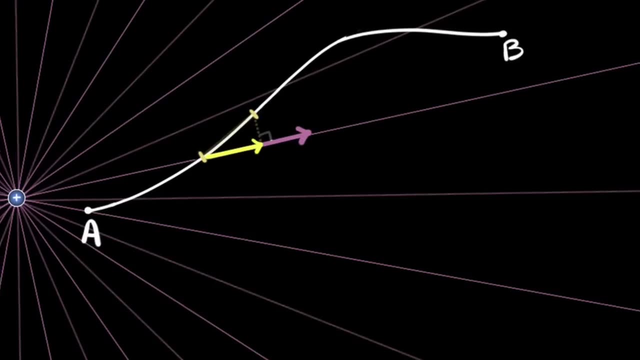 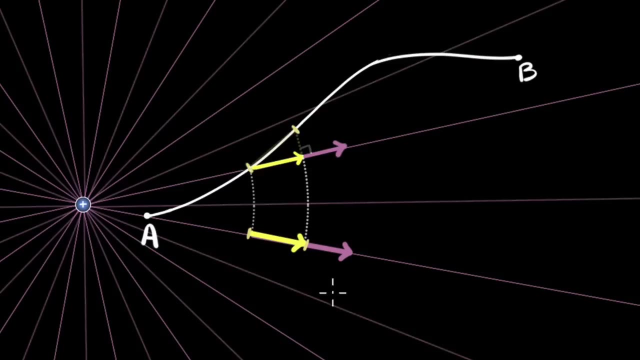 displacement in the direction, and we multiply these two, That's what gives you the work done in this tiny segment, right, Yeah? Well, now Feynman argues that that work done is exactly the same as the work done in moving the unit charge from here to here along this field line. 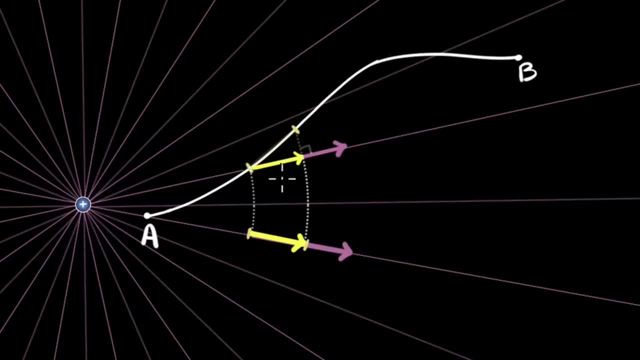 And let's see why: Because this force is the same as this force, because the force is radially symmetric, the field is radially symmetric, we are at the same distance from the charge, So these forces are exactly the same. And, look, we are taking the exact same displacement. So of 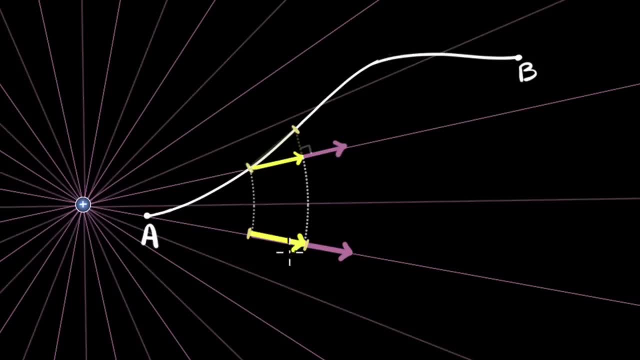 course the work done will be the same here. Okay, And now Feynman says: well, let's consider another such section. So let's consider another such section. So let's consider another such section. So let's take the work done somewhere over here, And if we calculate the work done over there, 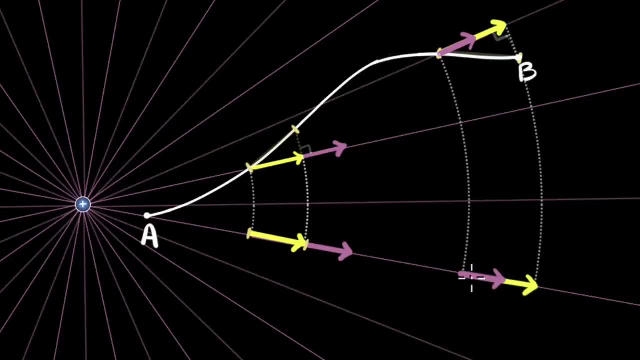 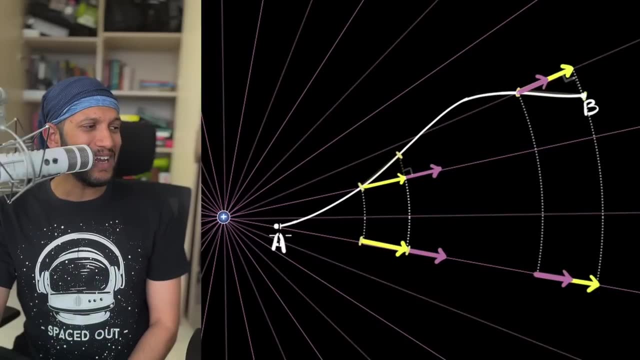 again, we can say: the work done in that section equals the work done in moving that charge from here to here along this field line. So look at what Feynman is saying. I can divide this into tiny, tiny sections, And what I will find now is that, from similar argument, the work done in each 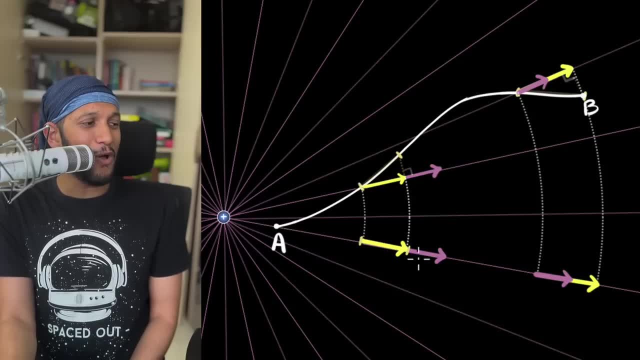 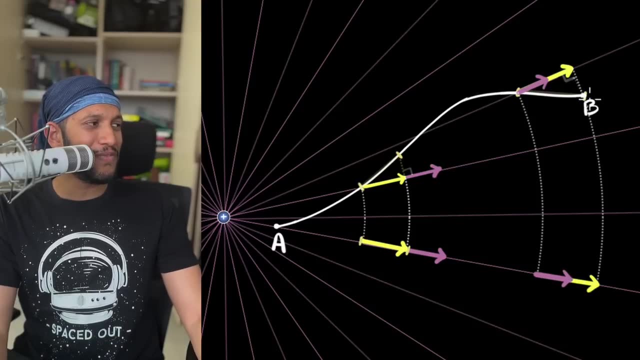 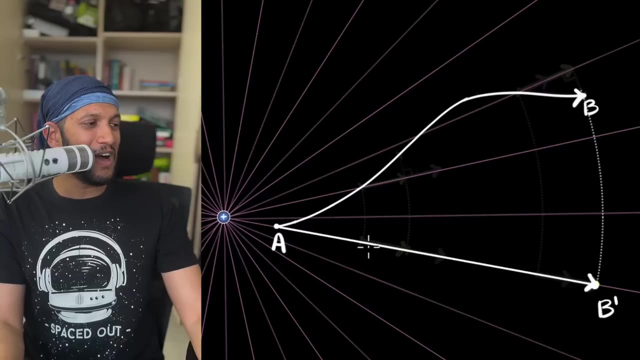 of this section exactly equals the work done in moving the charge along this field line. In other words, in moving the charge from here to here along this path should be exactly the same as the work done in moving that point charge from here to here along this field line. 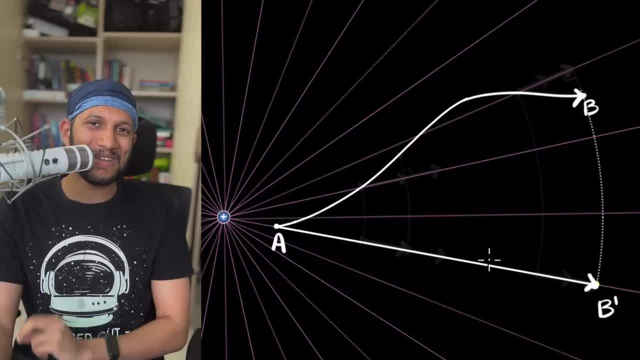 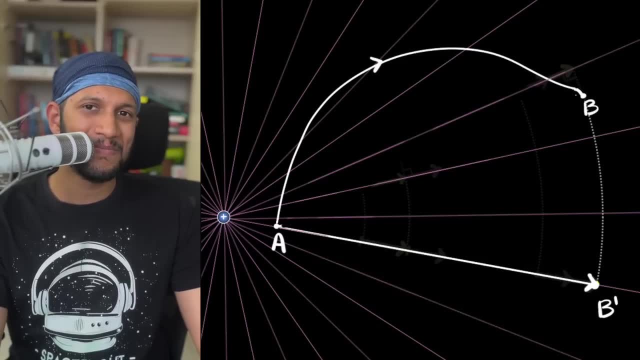 All because of the fact that the forces are symmetric. Since this is a random path, I could have chosen this path and I would have gotten the same answer. So any path you take, the work done should be the same as the work done in going from here to here. 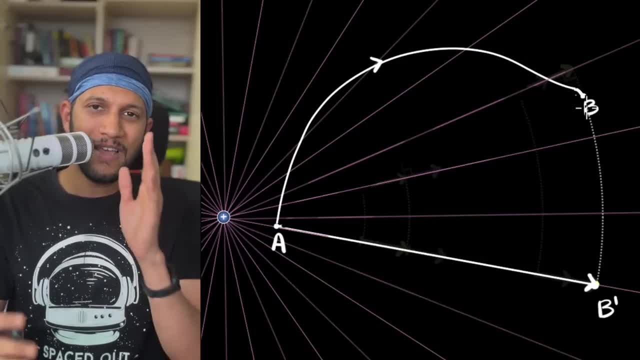 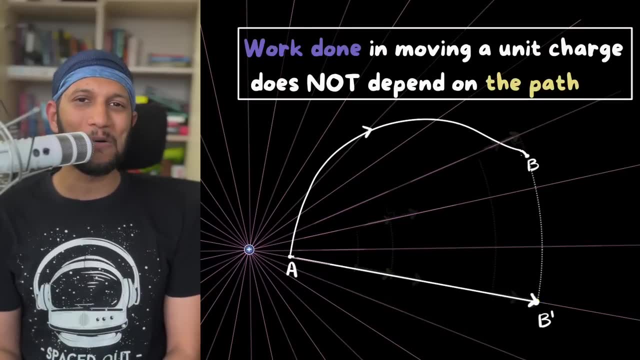 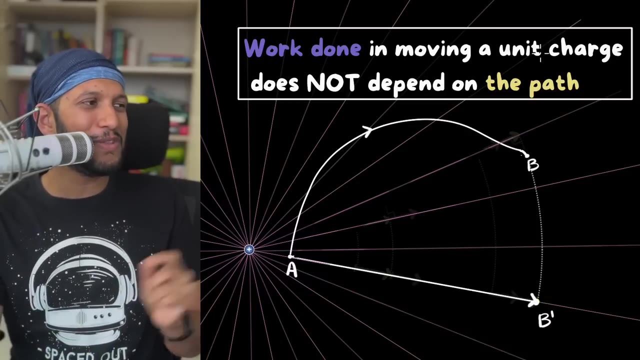 which means the work done should always stay the same between these two points. The work done should not depend on the path taken. Wow, The simple fact that the field is radially symmetric means the work done in moving the unit charge does not depend on the path taken. 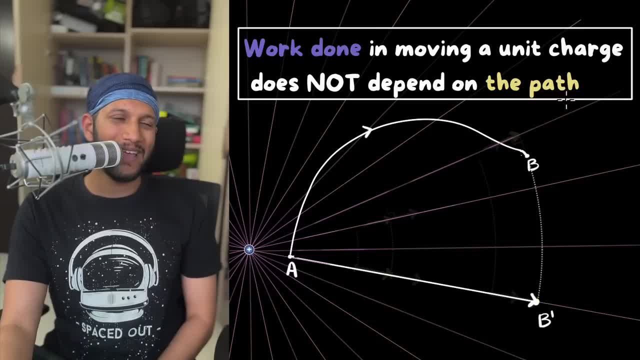 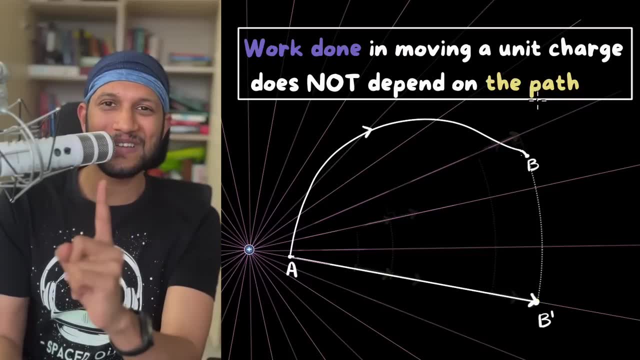 That's amazing. And now Feynman says: write that in the form of equation, Mahesh. But again, how do I write this statement as an equation? Here's how says Feynman: This is the last step, okay. 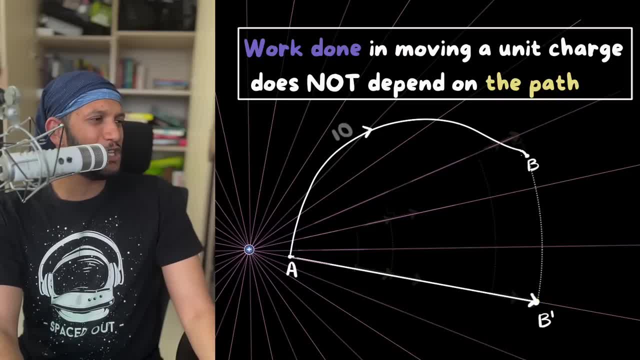 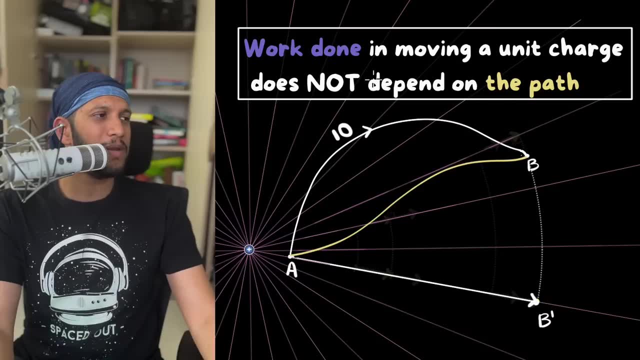 He says: let's assume that the work done from here to here was. some say 10 joules or 10 units. Now if I take some alternate path, the work done from here to here should also be 10 units, because the work done does not depend. 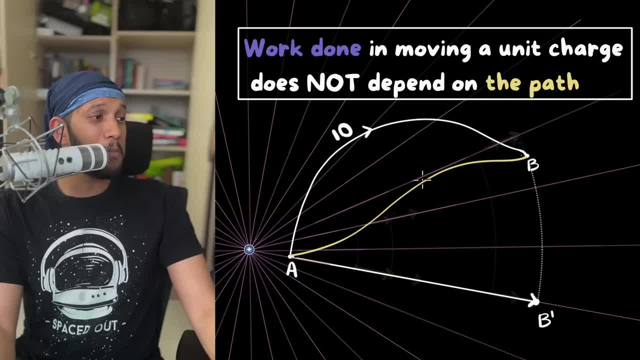 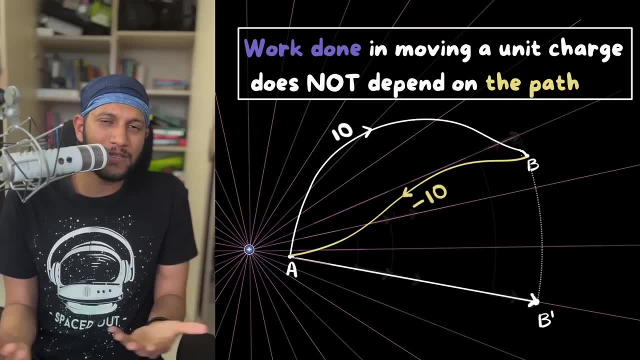 upon the path taken. right, Which means the work done to go from B to A in the exact opposite direction should be negative 10,. right, Because now the displacement will everywhere be in the opposite direction. giving you a negative answer, Yes. 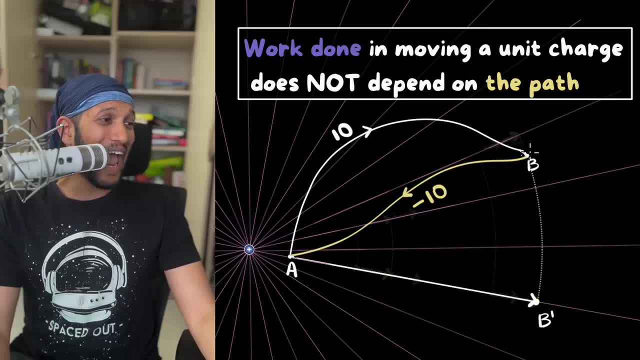 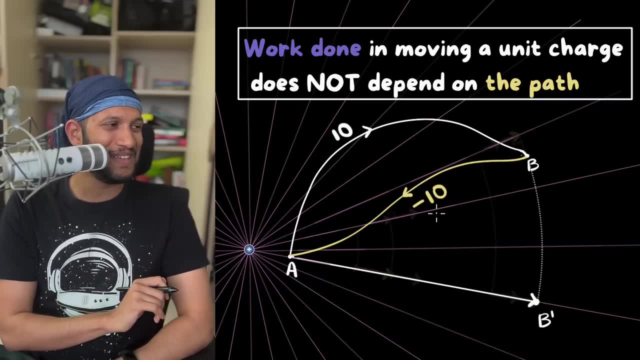 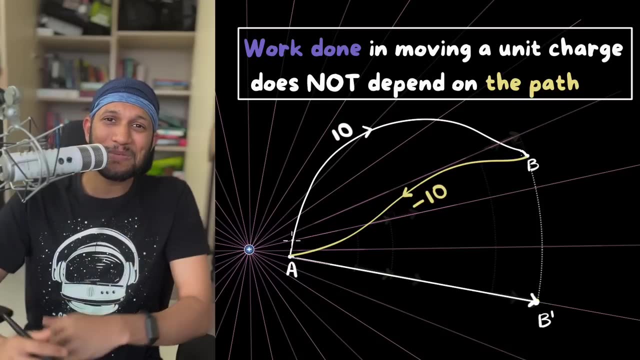 This means the work done to go from A to B and B to A should be zero Plus 10 minus 10 should be zero. In other words, the fact that the work done does not depend on the path automatically means the work done in a closed path must be zero. 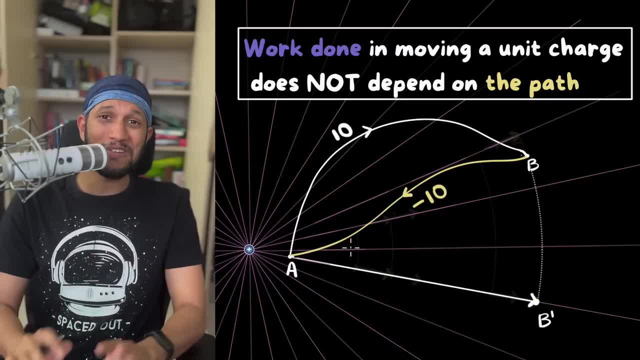 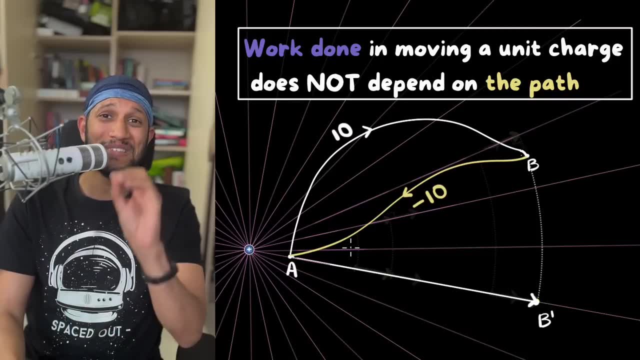 And since we took this path randomly, this should be true in general. It doesn't matter what path I choose, as long as it's a closed path. the work done must be zero Zero. That's what this statement actually means, And now we can write that. 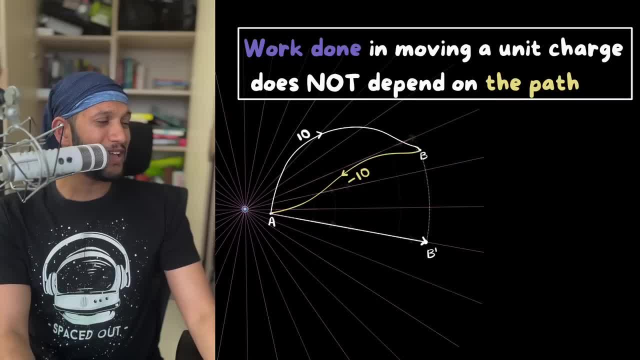 Yes, we can write that. If I minimize this work done in a closed path, How do we calculate the work done? Well, work done is the integral of F, dot, DL And, by the way, force on a unit charge is basically the electric field. 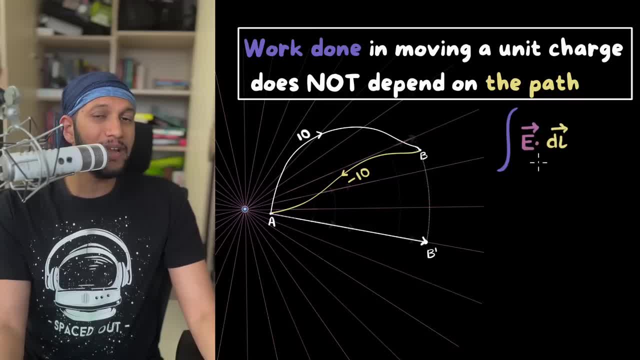 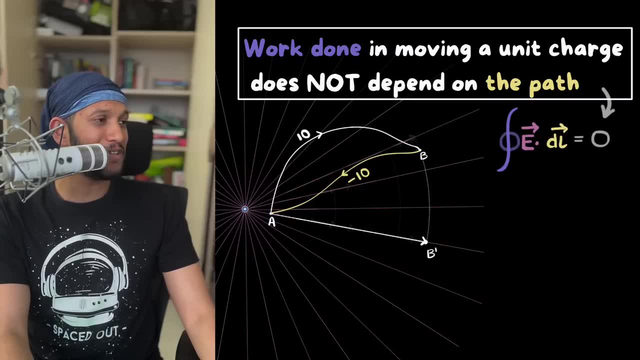 So the work done on this point charge is basically the integral of E, dot, DL And in a closed path. so to write the closed path, we put a circle on the integral mentioning it's a closed path and it says that it should always be zero. 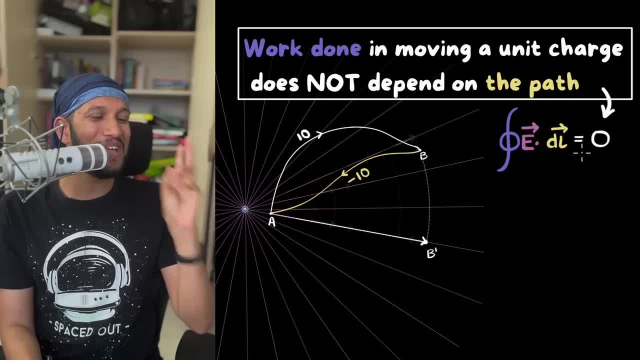 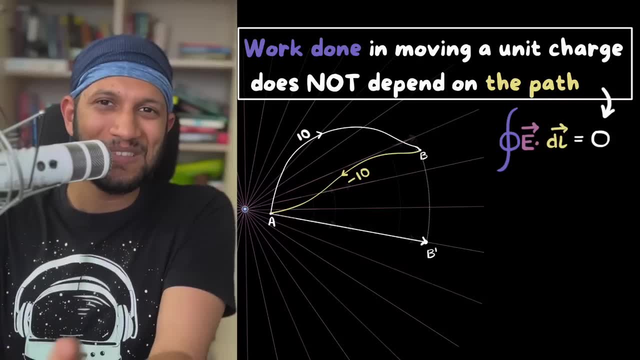 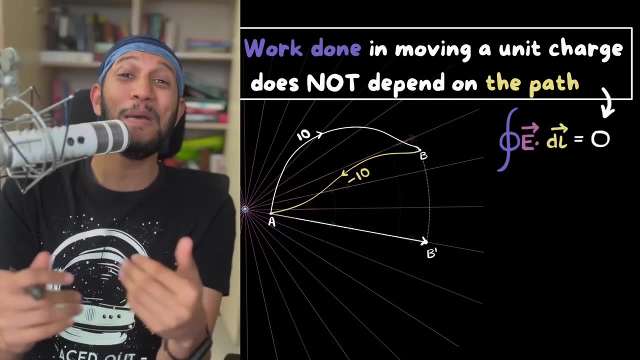 This is a part of Maxwell's third equation. So if you put it all together, the fact that a point charge gives out a radial field means work done, is path. independent means work done in a closed path, is zero, means integral of E, dot DL. 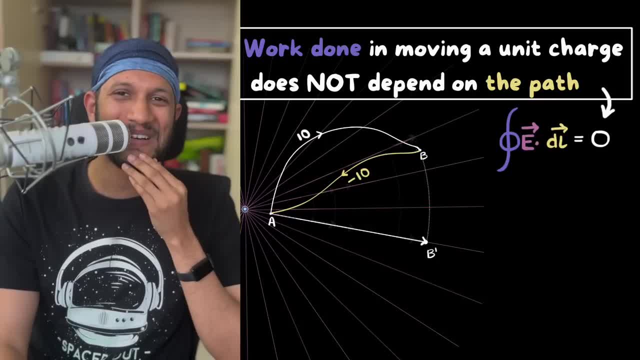 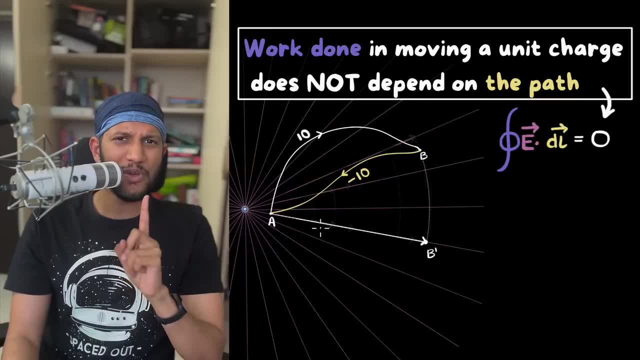 in a closed path should be zero. Isn't this amazing? Look at how we are progressing, wow. But wait a second, Feynman, This is true only if you have a single charge, because only then you will have a radial field. 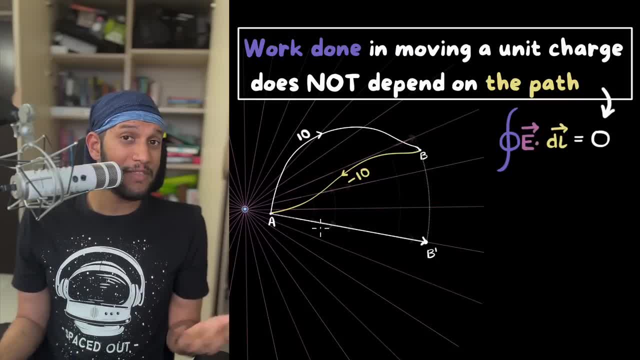 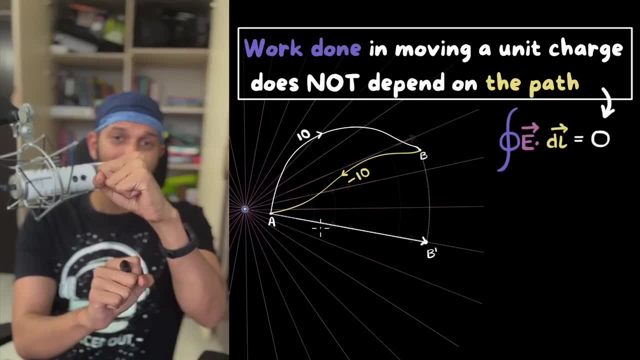 If you have multiple charges, you will no longer get a radial field, and this will not be true, right? Well, Feynman says no. He argues that if you have, say, two charges and you calculate the work done in a closed path, 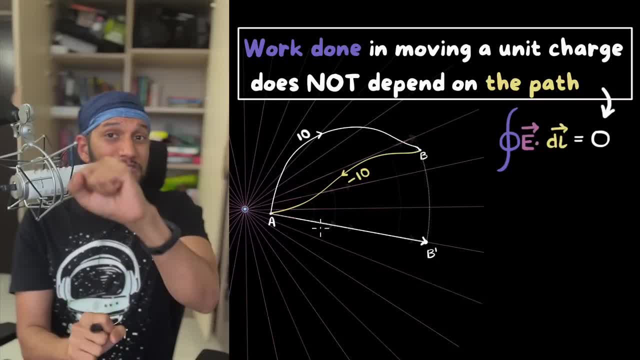 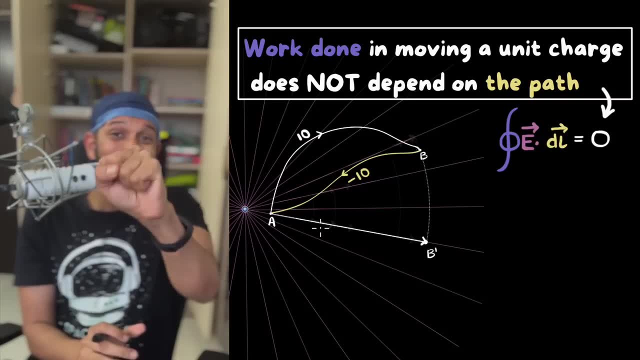 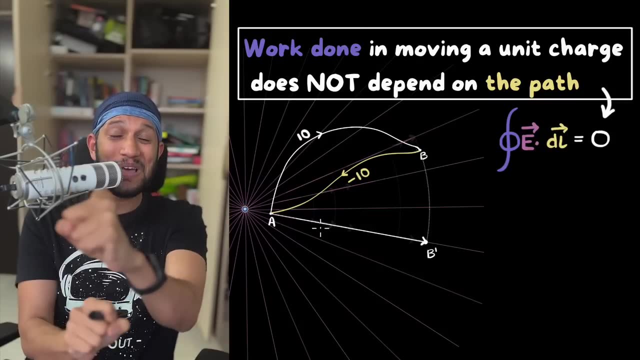 that total work done can be written as one. It has work done due to the first charge plus the work done with the second charge. superposition principle And since the work done due to the forces of each charges will individually give you zero, the work done due to the two charges combined together. 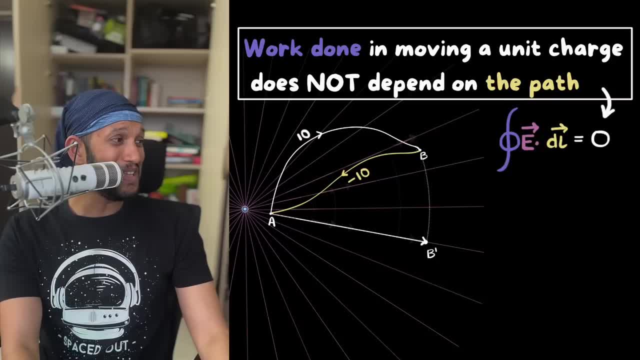 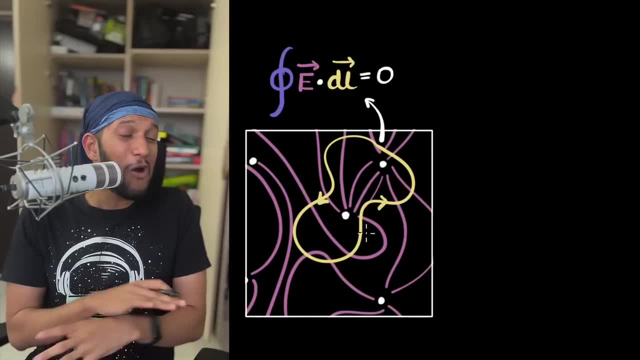 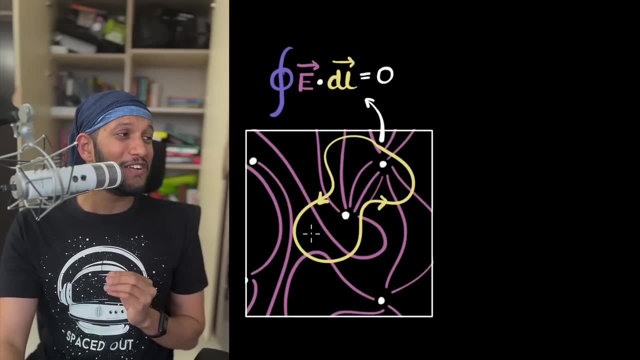 must also give you zero. What this all means is that it doesn't matter how many charges you have. it doesn't matter how complicated or how crazy the field lines are In a closed loop. when you move a charge, the work done must always be zero. 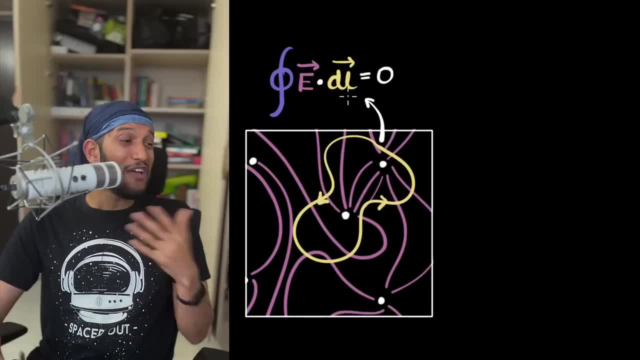 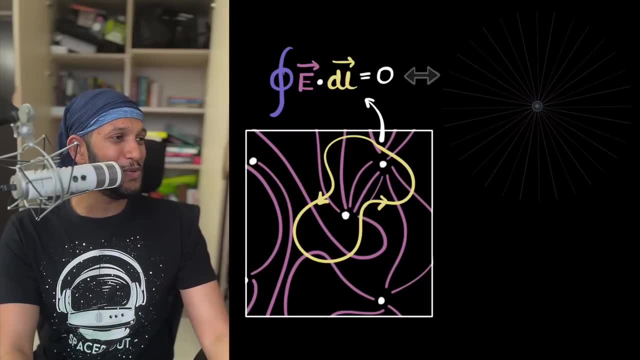 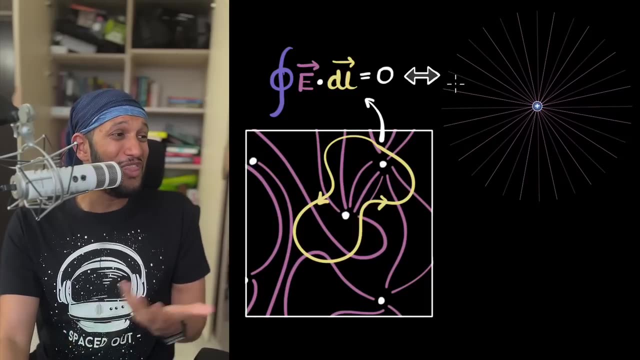 This is the beginning of Maxwell's third equation, And I find it so fascinating because, at the heart of it, what is this equation basically saying? That each individual charge is giving out a radial field. That's what it's saying. These two statements are synonymous. 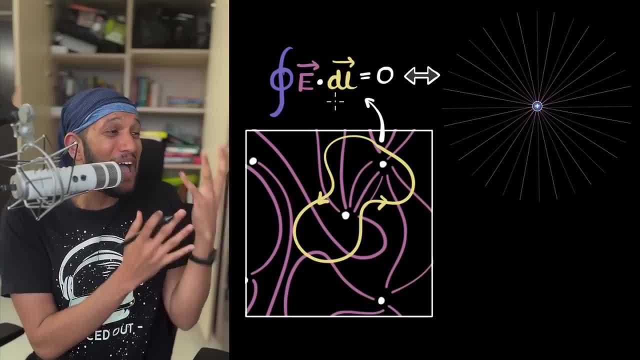 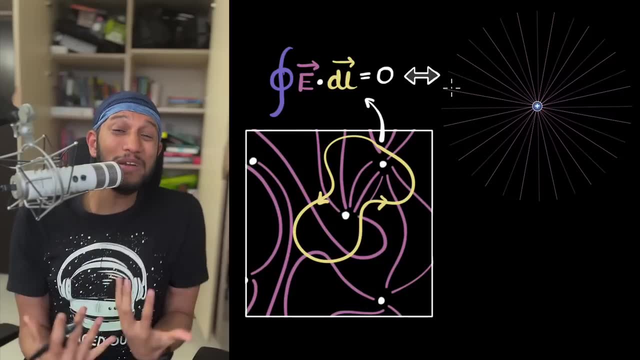 That information is packed in this equation. How elegant is that. To the uninitiated, this wouldn't make any sense. They would say: what is this? but now you and I understand that these are the two same things. We are communicating in a different language. 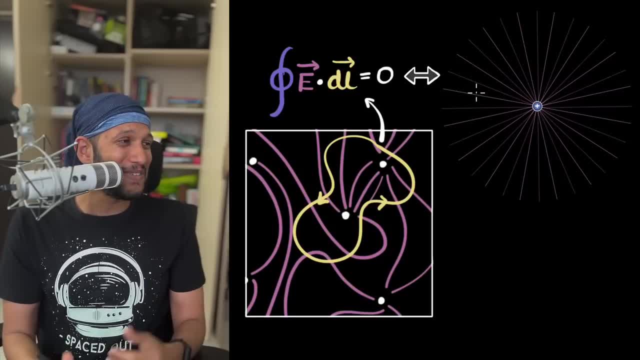 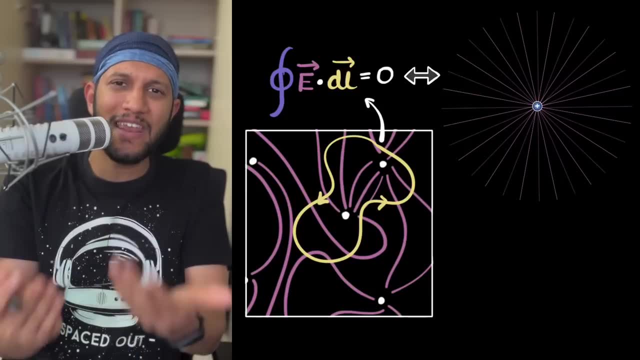 Oh man, That's why Maxwell's equations are so awesome. If electric fields don't do any work in moving a charge in a closed path, they do not transfer any energy In electrons, for example, in moving it in a closed path- right. 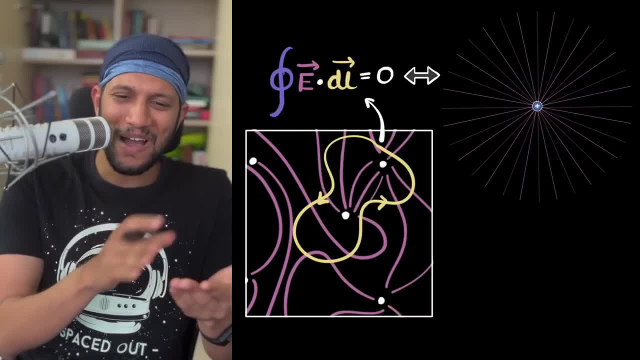 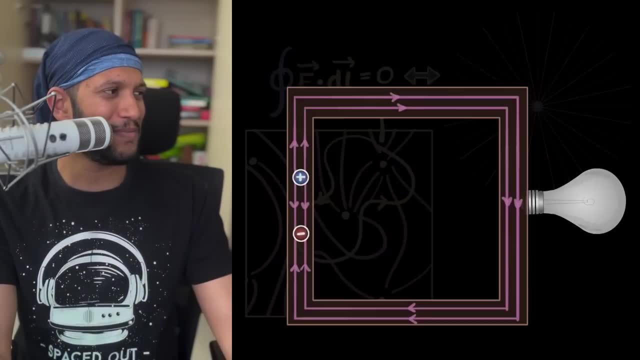 But then how do circuits work? Because in circuits, Electric fields are moving the electrons in a closed path and they are transferring energy, isn't it? And Feynman says not quite. If you look at the circuit carefully, what you will see is that it can make an electron say: go from here. 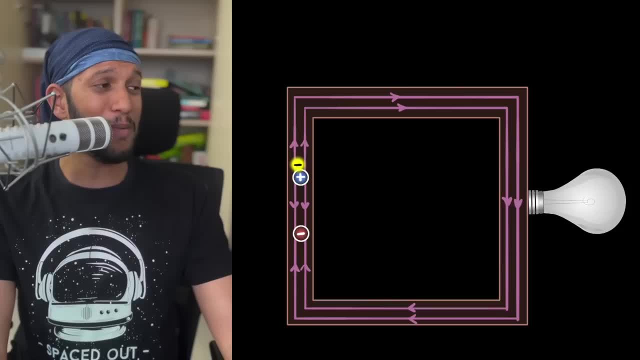 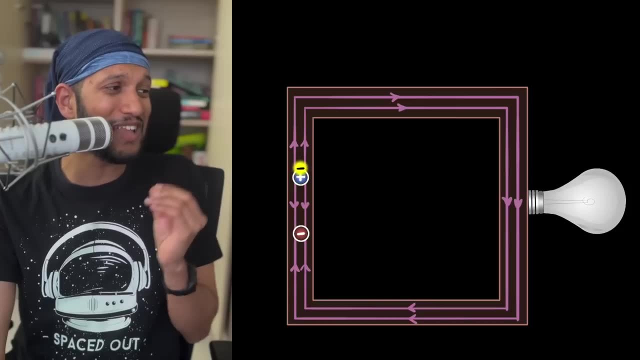 all the way till here, but it will not be able to make it go back over here. Look for the electron to go back. it needs to be pumped down. Something external has to pump it. This electric field will not be able to do it. 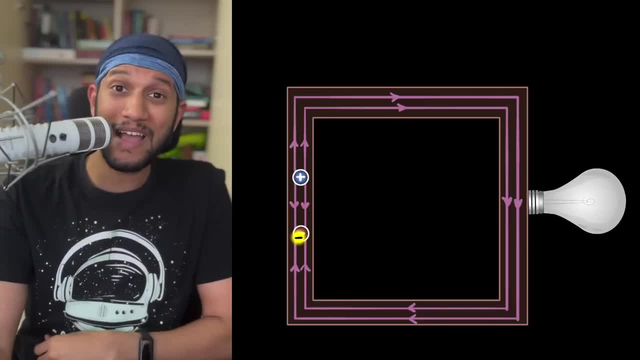 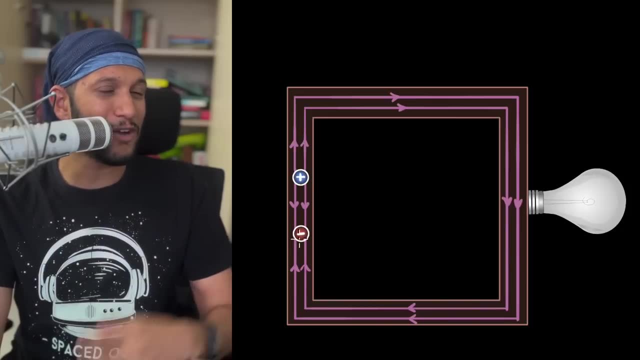 How do we do that, Feynman? How do we pump it down then? Well, we use chemical reactions, because in chemical reactions electrons can jump from one atom to another. So if we cleverly place these two atoms, set of atoms, separate, 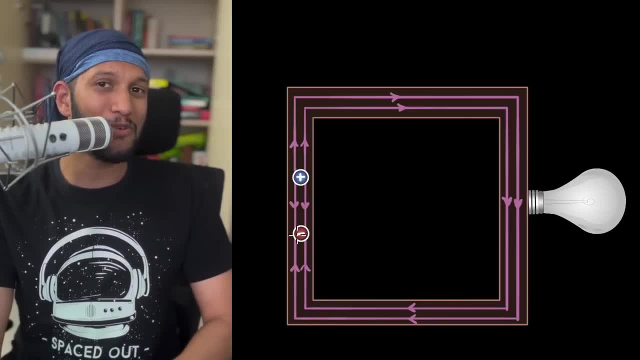 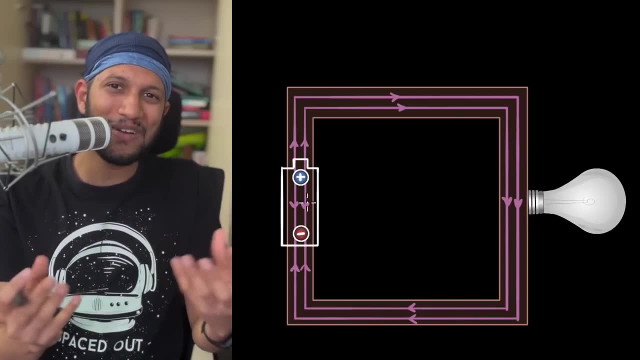 and have chemical reactions, then the electrons can pump from here to here, And that's exactly what we do in a battery. We have a couple of different electrodes, which basically means a couple of different atoms, and then you have chemical reactions where electrons are pumped. 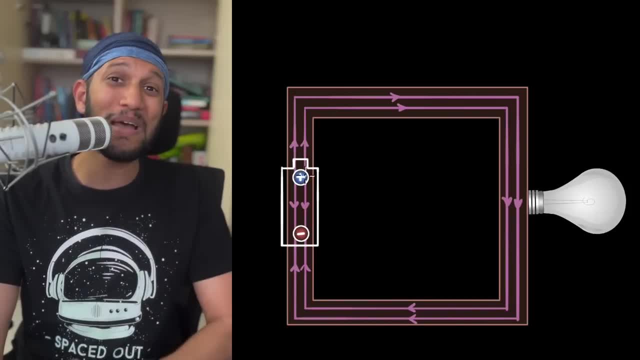 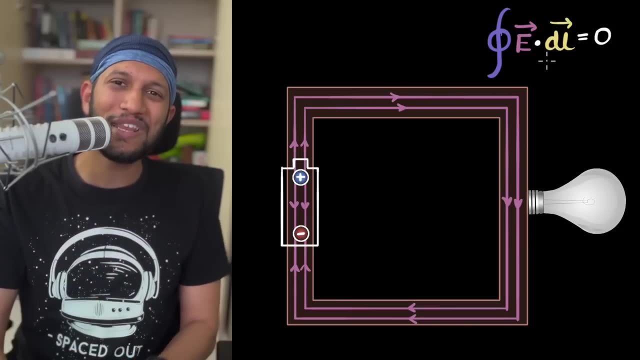 and that's how electrons keep going in a closed loop. because there's a battery, because we use chemical energy. We need batteries because closed-loop integral of E, dot, DL must be zero. Electric fields cannot transfer any energy in a closed loop. By the way, if you have solved multi-loop circuits, 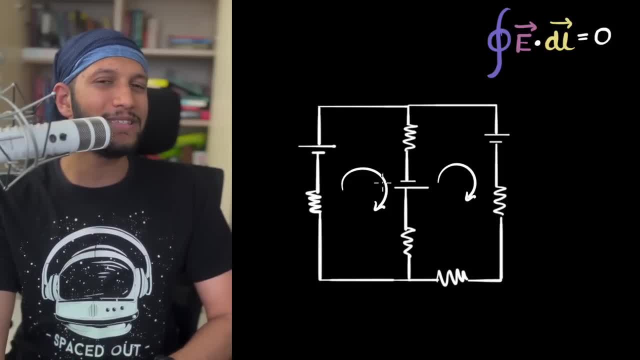 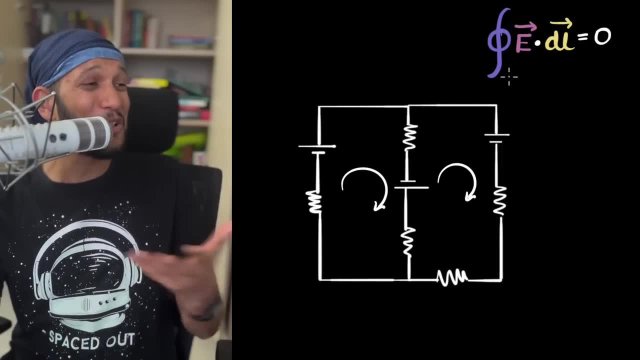 you've probably done this loop analysis where in each loop you add up voltages and you say that equates to zero. Guess what that is. You say Kirchhoff's law, but that's the same thing. Closed-loop integral of E dot DL is zero. 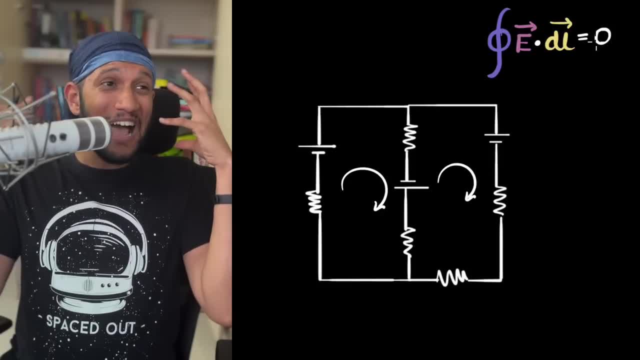 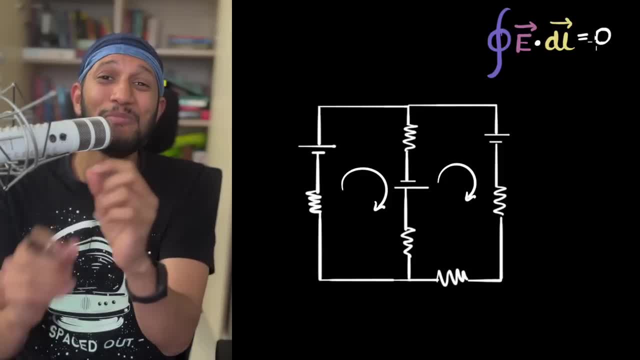 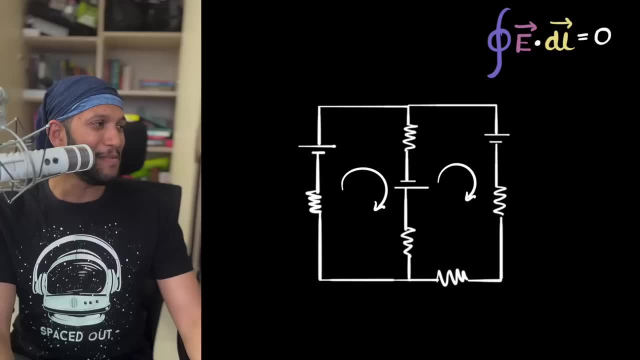 It's all coming from one atom. It's all coming from one atom. It's all coming from one thing: that a unit, a single charge, produces radial field has such far-reaching consequences. Whoa. But Feynman now says Mahesh. this equation is incomplete. 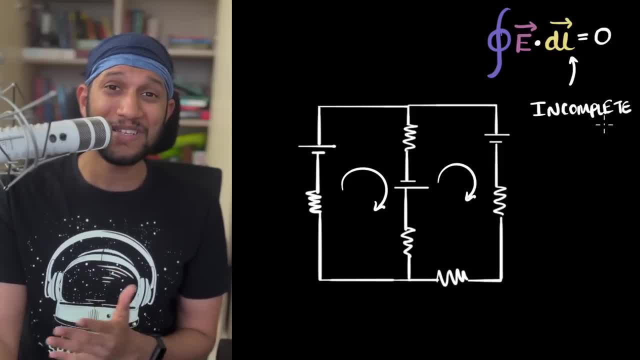 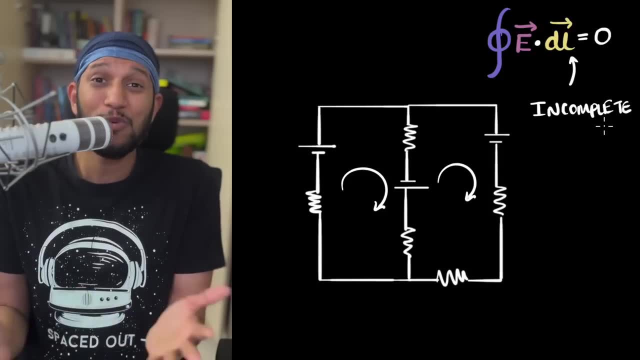 I'm like, first of all, thank God that this equation is incomplete, because if it was the complete equation, the only way to power up circuits would be using batteries, And we wouldn't be able to do that in large scale. We can't practically build large, factory-sized batteries. 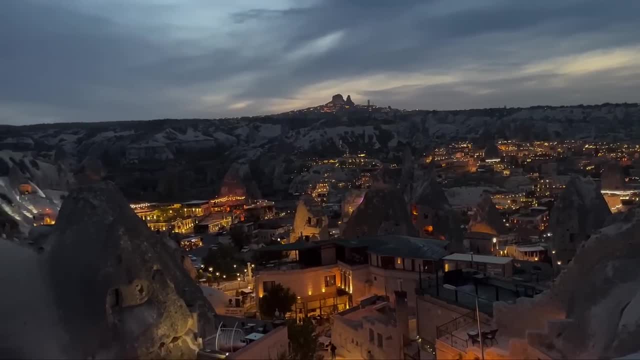 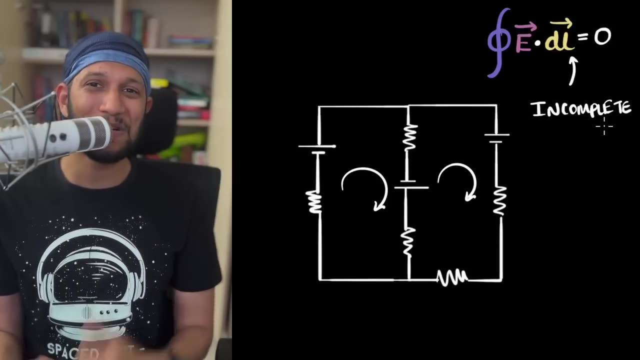 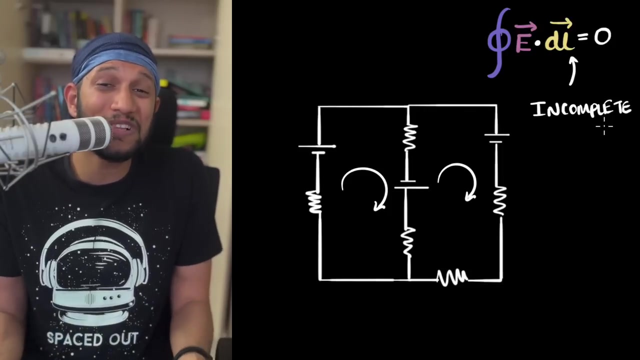 We wouldn't be able to light up cities. The world would have been a dark place. The reason why we have power worldwide is because that equation is incomplete. Feynman, how can that equation be not complete? We just looked at it in the most general case, right? 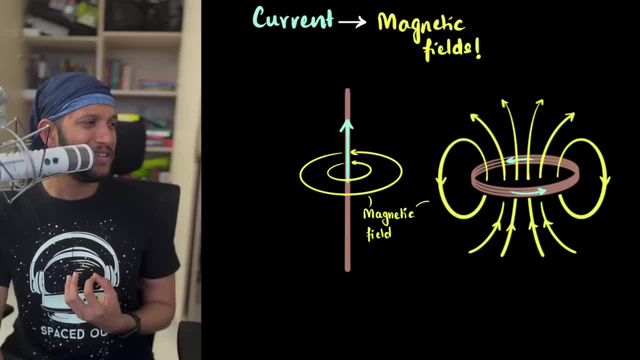 Well, Feynman says no, we didn't. You see, in the 1800s we realized that the electricity and magnetism are linked, That electric currents themselves can generate magnetic fields. For example, a straight wire will give you looping fields. 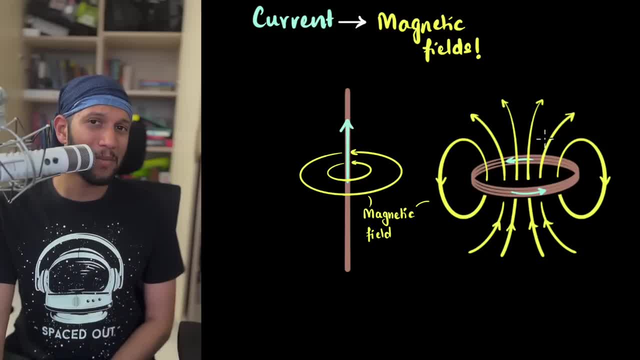 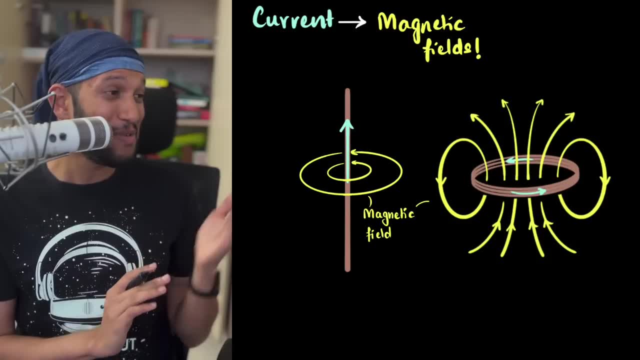 and a looping current will give you magnetic fields that resemble a bar magnet, And we did a lot of experiments. that eventually leads us to Maxwell's fourth equation, which is a story for another day. But for our sake, there's one scientist named Michael Faraday. 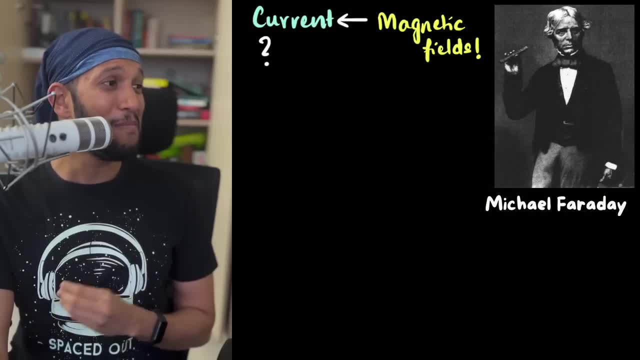 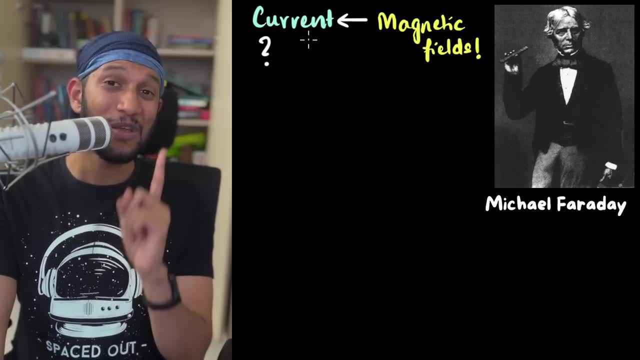 who was thinking whether the reverse would be possible, whether magnetic fields can generate electric currents? because even he was thinking about it. Can we generate electricity without balance? Can we generate electricity without batteries? So how did he test it out? Well, simple. 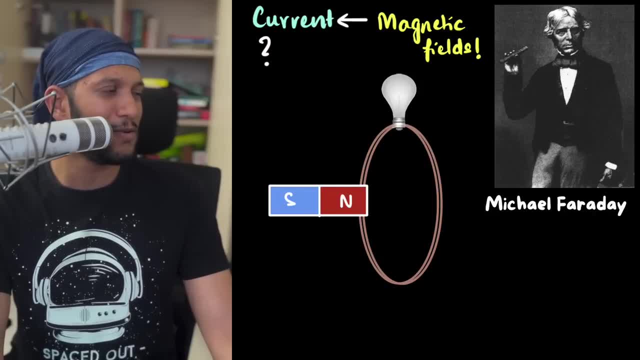 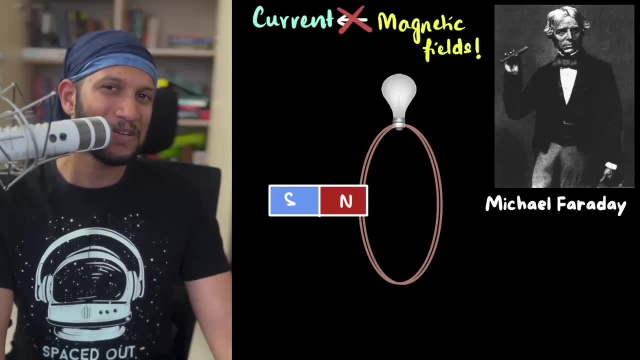 He kept a magnet close to a coil and he did a series of experiments. The simplest one is he kept a magnet close to a coil and saw if there is a current. Well, there wasn't a current, So he realized magnetic fields cannot generate electric currents. 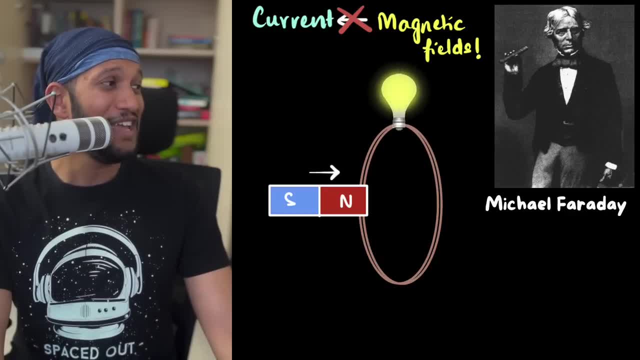 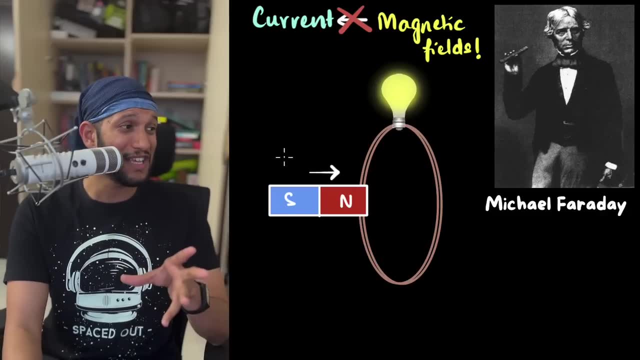 However, you probably already know that when he moved the magnet, he saw that there was electricity generated, but only as long as the magnet was moving. So look at this. So look, says Feynman, we have a way of generating electricity without a battery. 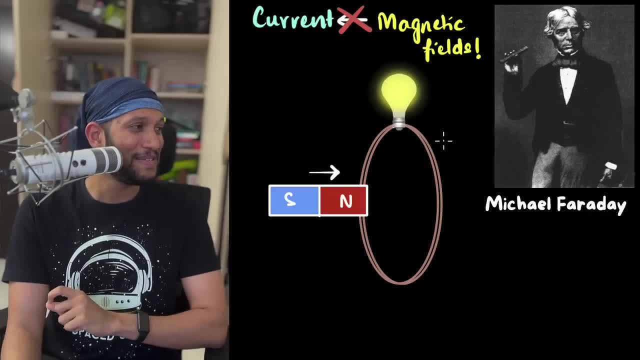 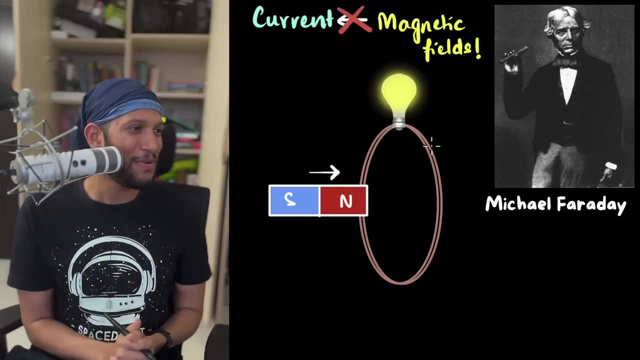 So something else must be going on and therefore that equation is incomplete. But, Feynman, what does it mean? Why is this happening And how can we use this to complete the equation? This is it, folks. This is the final step. 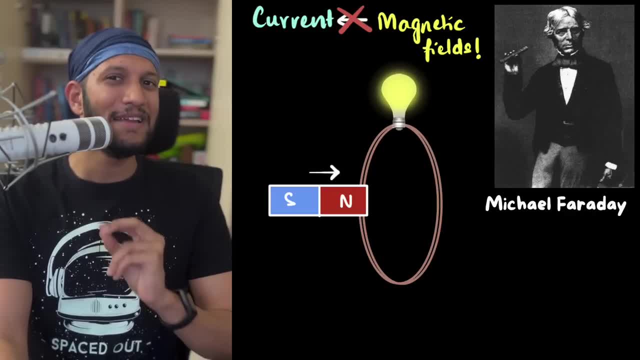 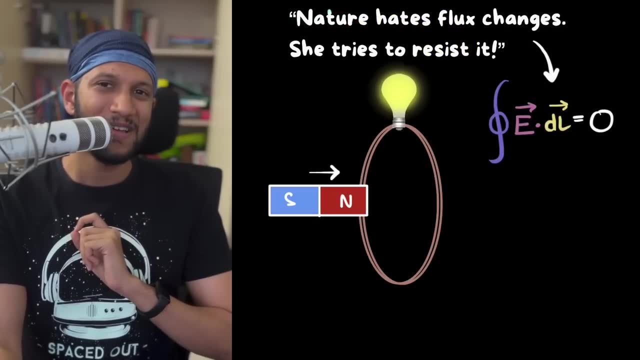 What this all means. the reason why this is happening is because there's a secret that nature has been hiding from us for quite some time, but this reveals it. Nature's secret is that she hates flux changes Whenever there's a flux change. 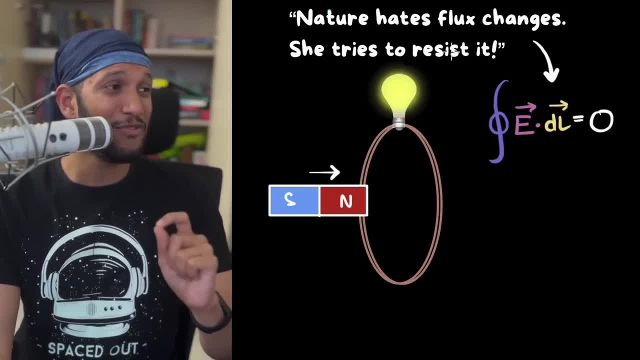 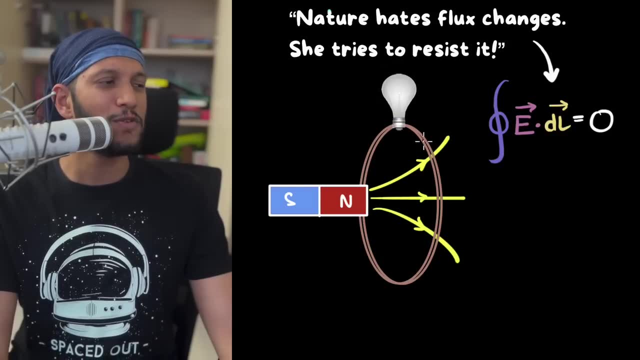 she tries to resist it And then that happens And if you can incorporate that part in this equation, we would have completed it. So, when the magnet was not moving and was kept close to the coil, because there was some magnetic field passing through the coil, 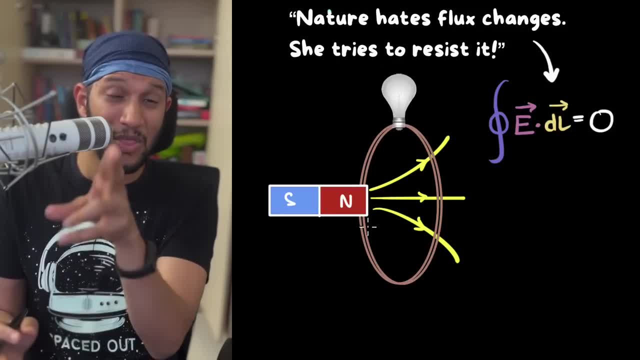 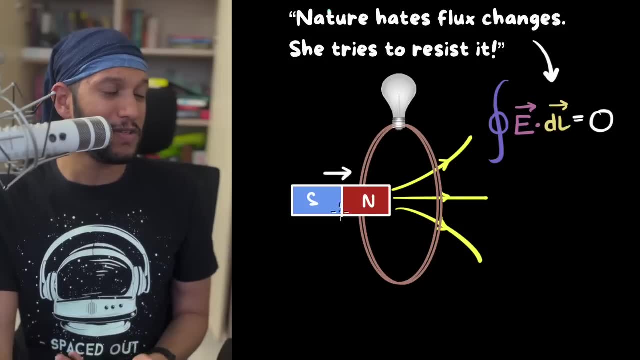 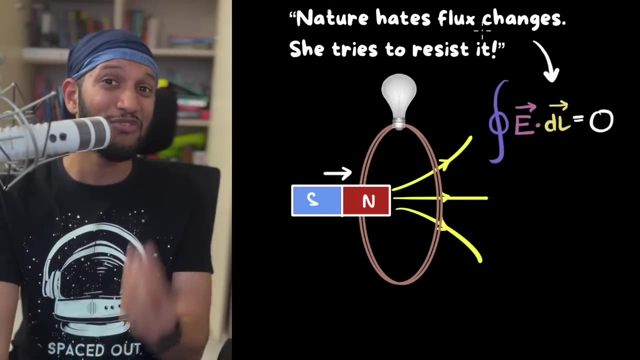 which means there is some magnetic flux through the coil right Now. look at what happens when you move it closer. While you're moving it closer, the magnetic flux through the coil increases And nature hates flux changes. But you can ask: well, why does that happen? 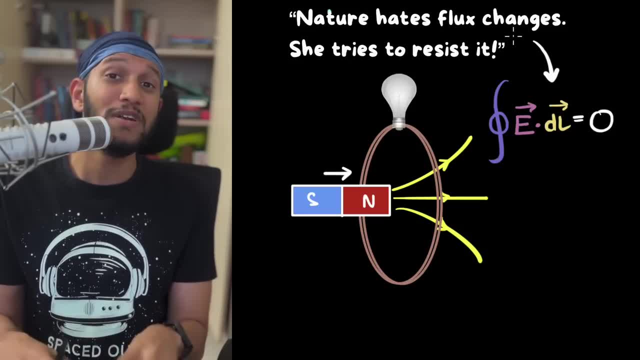 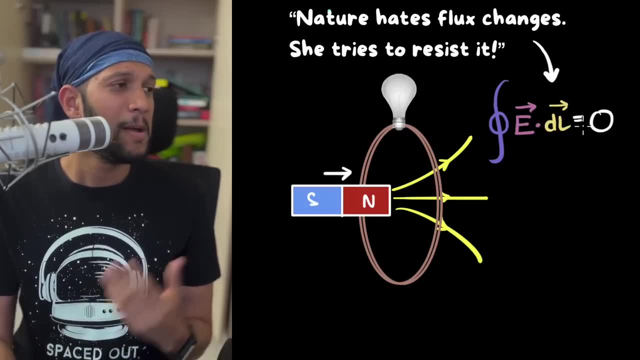 Why does nature hate it? Well, Feynman says that's like the most fundamental rule which we're going to incorporate in the Maxwell's equation. You can't ask why? to every single thing. That's the most fundamental thing. But now the question is: 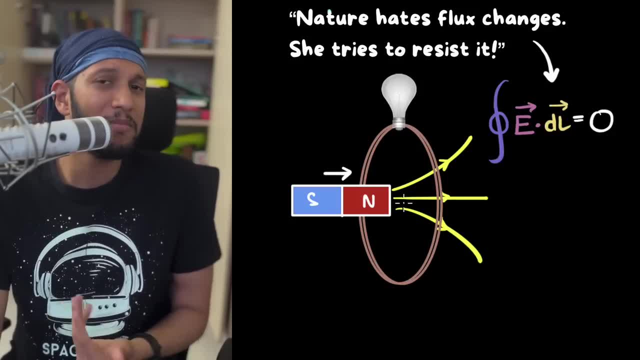 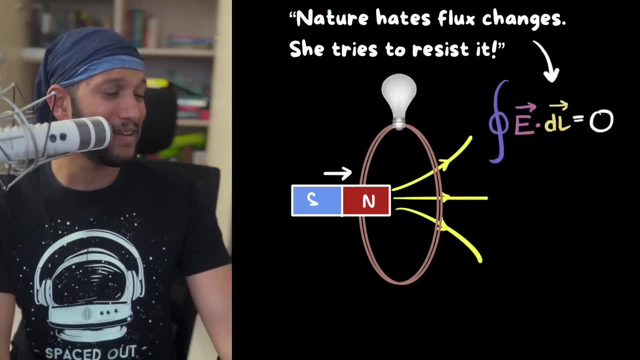 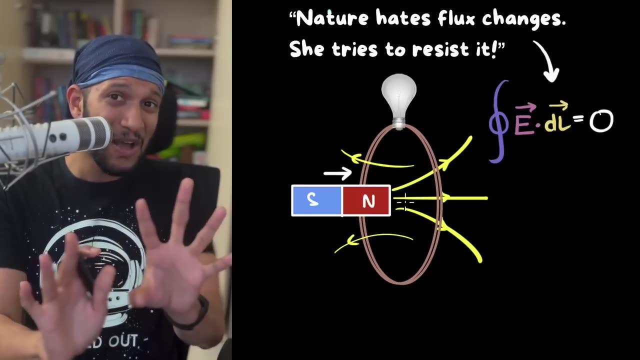 how does she resist it? How can she ever resist a moving magnet? Well, by repelling the magnet. The coil repels the magnet and to do so, it will generate its own magnetic field in the opposite direction. That's how it will resist. 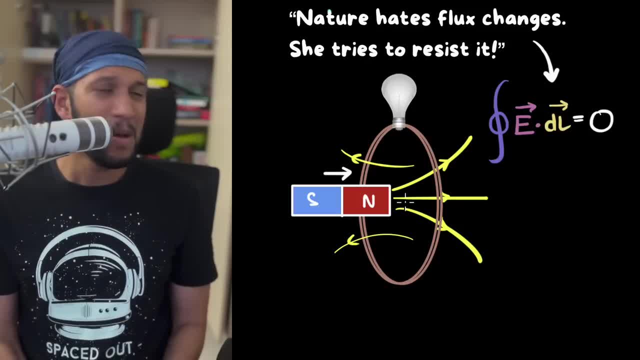 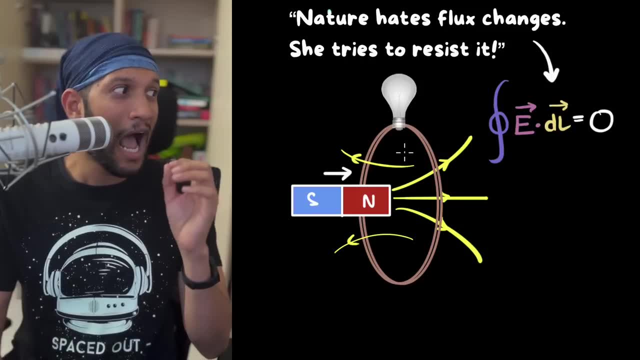 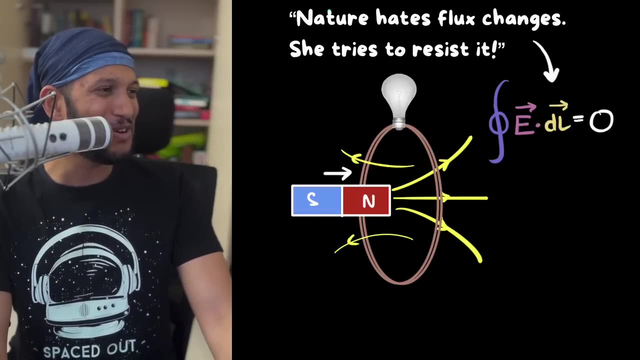 the changes in the flux by repelling the magnet. But, Feynman, that's a piece of wire. How can a piece of wire generate a magnetic field? By generating a current. That's the reason, that's the core motivation for nature to generate. 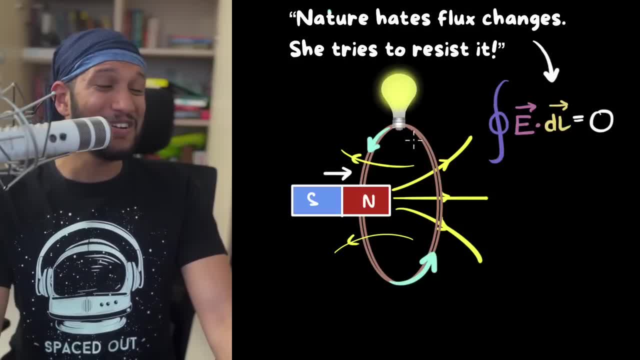 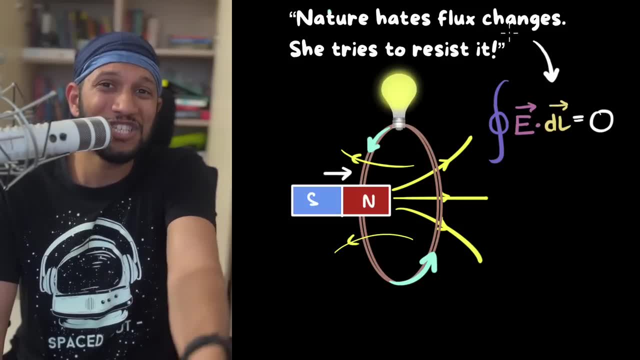 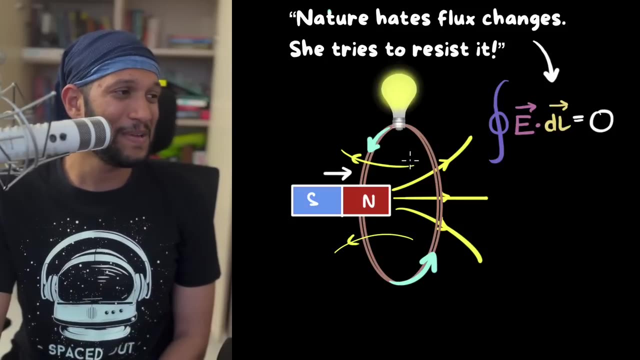 the current. That's why it generates the current: so that it can generate a magnetic field, so that it can repel the magnet, so that it can resist the flux change. And in doing so, we have now a current generated in the coil. 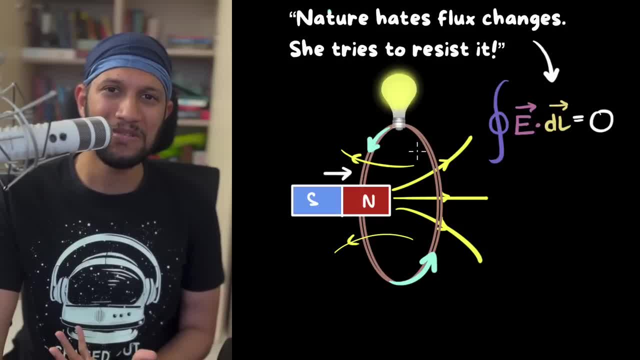 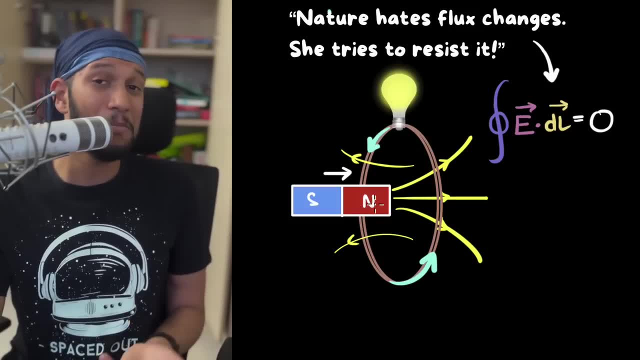 But, Feynman, where does that current come? where does the energy come from? Like the energy has to be conserved, It should come from somewhere, right? Well, in trying to resist the magnet, it's slowing the magnet down. 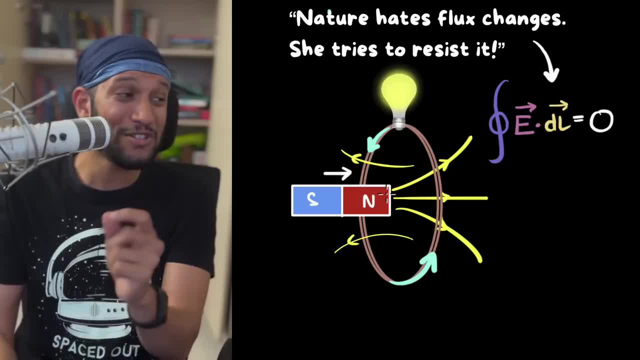 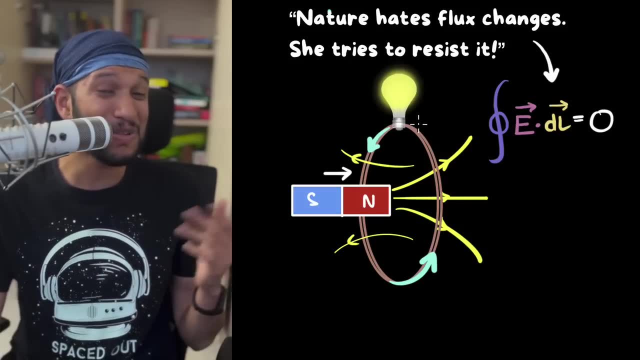 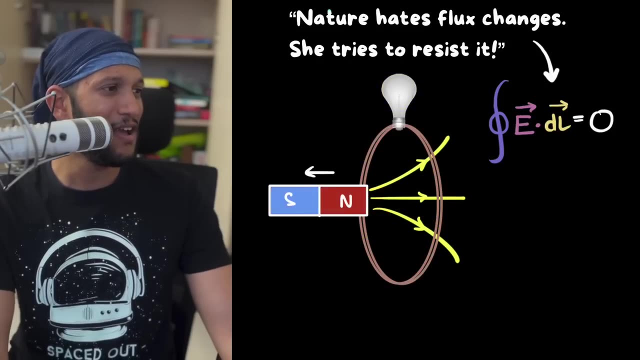 It's sucking its kinetic energy. The kinetic energy of the magnet is being converted into electrical energy. That's what's going on. And now you'll understand this. What if you were to move the magnet away from the coil? Well now, if you move the magnet away from the coil, 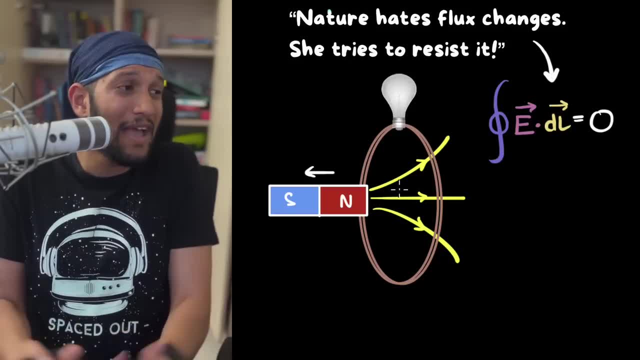 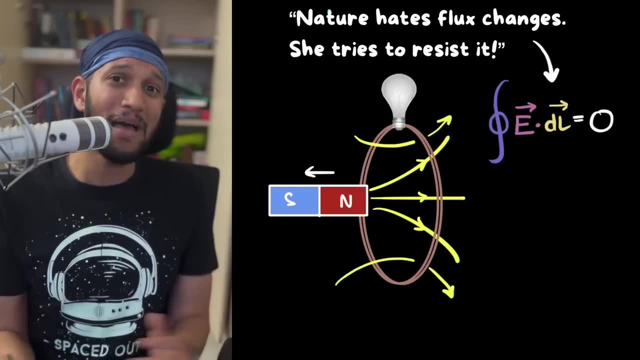 again there's a flux change, The coil will say: I don't want you to move away, I don't want the flux to decrease. If you were to increase the flux to do so this time. it'll try to attract the magnet. 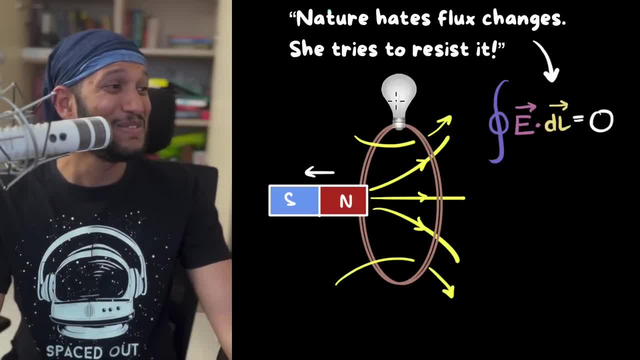 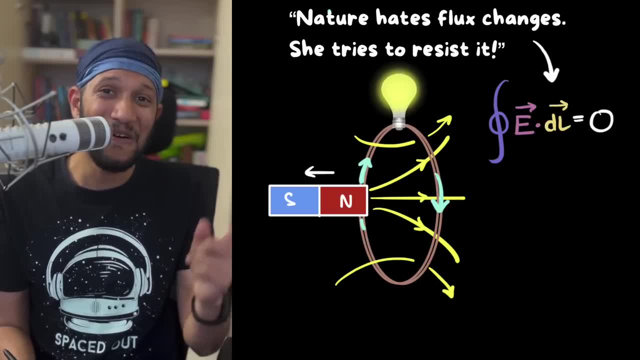 Because its job is to slow down that magnet, make sure it doesn't move. So this time it tries to create the magnetic field in the opposite direction and for that it will create the current in the coil in the opposite direction. And finally, Faraday. 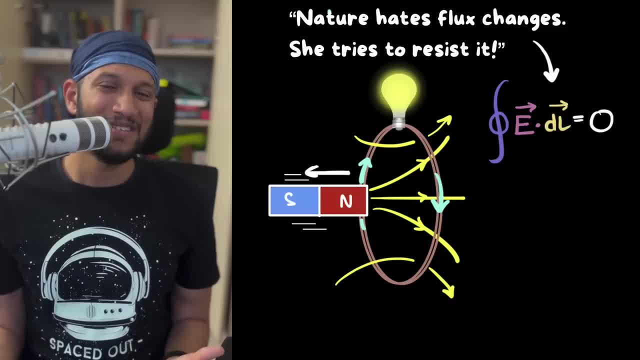 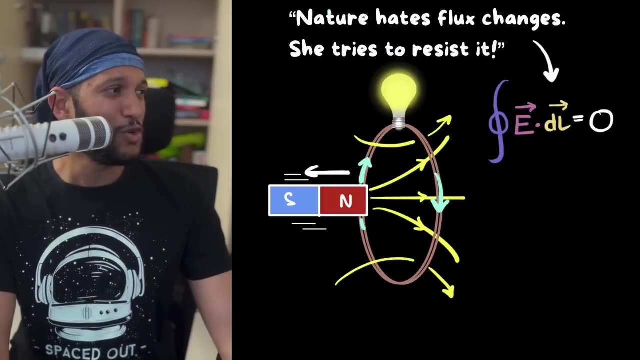 wondered what happens if I move the magnet faster. Well, if you move the magnet faster, then the flux change. the flux changes quicker, Nature hits it even more, And she tries now even more desperately to stop that magnet, and to do so. 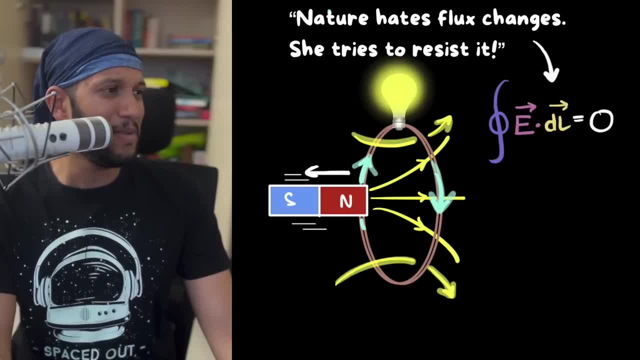 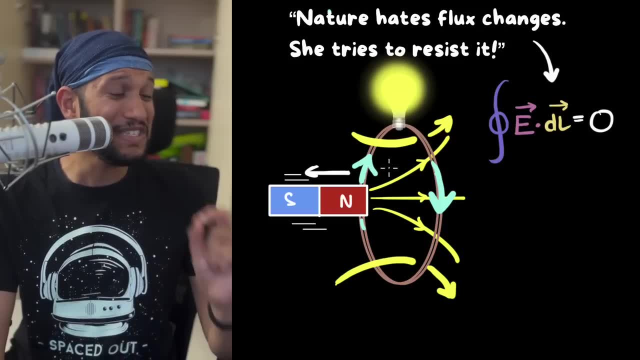 she tries to create her own stronger magnetic field by generating more current, by generating more energy. So can you see right from this experiment that the energy that is generated in this coil is equal to how quickly the flux changes, The quicker the flux changes. 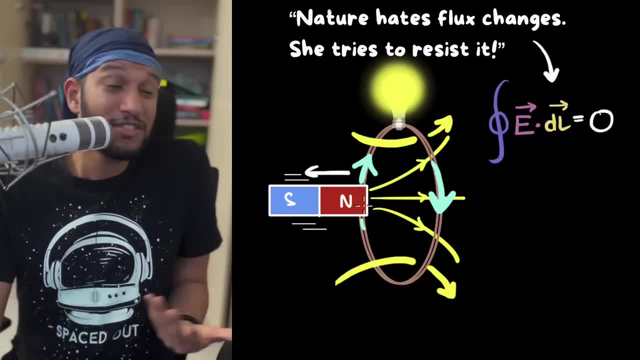 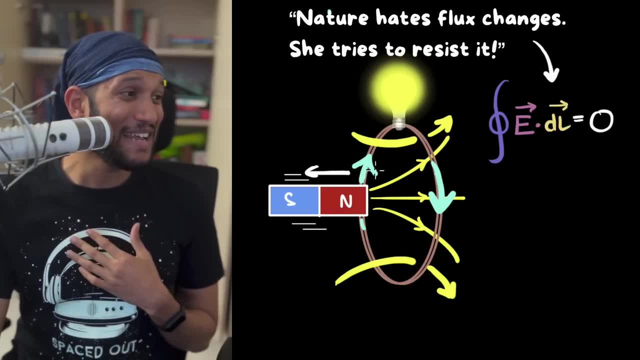 more the energy generated in this coil. If the flux doesn't change at all, there is no energy generated in this coil. But what's important for us is that if the electrons are moving, then there must be an electric field. Something must be. 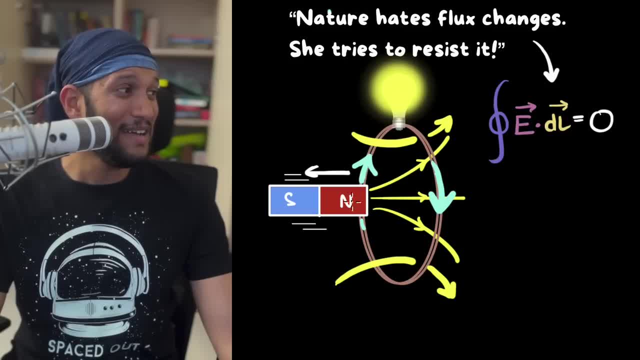 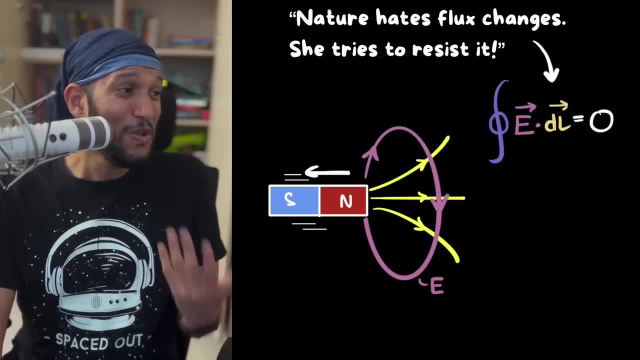 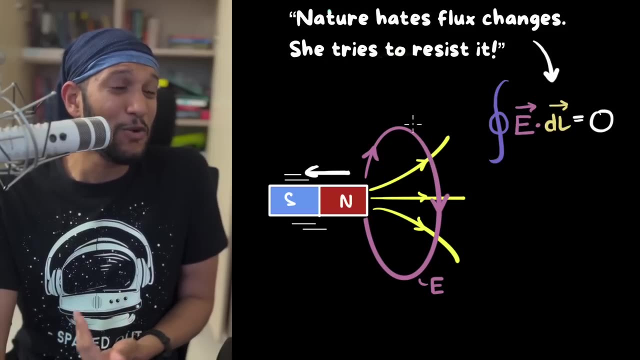 pushing that electrons, So there must be an electric field, and since there are no batteries over here, that electric field must truly be looping over here. So look, we have created a looping electric field And now, when it moves, the charges in this closed. 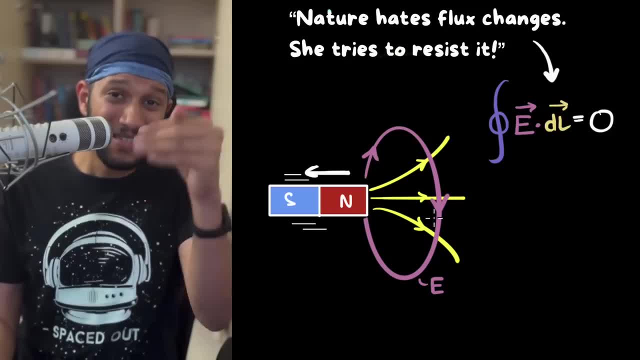 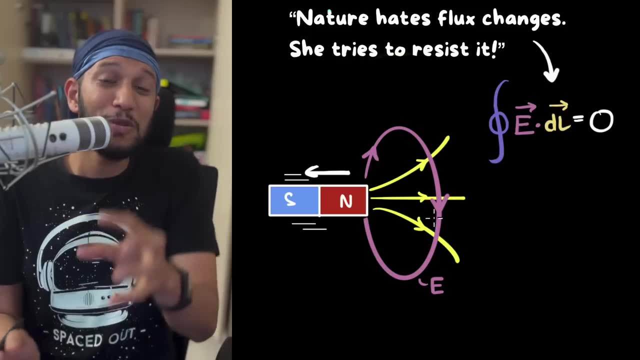 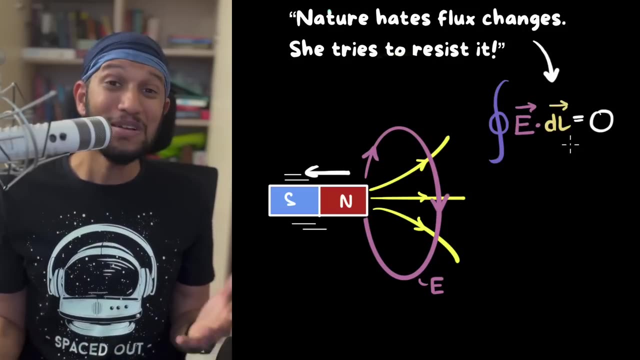 loop. it no longer does zero work. Now it does some positive work. Because of that, it was able to transfer energy into the electrons and to the bulb, Which means now closed loop. integral of E, dot, T, L is not zero. How much? 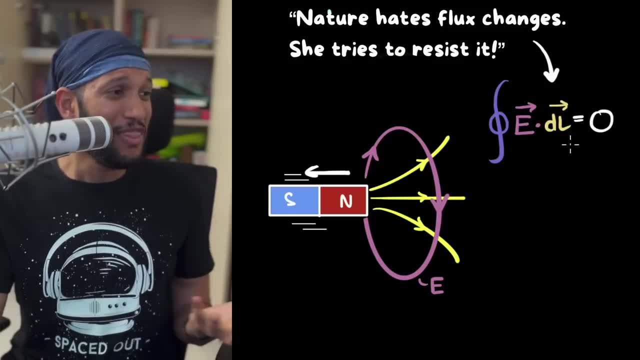 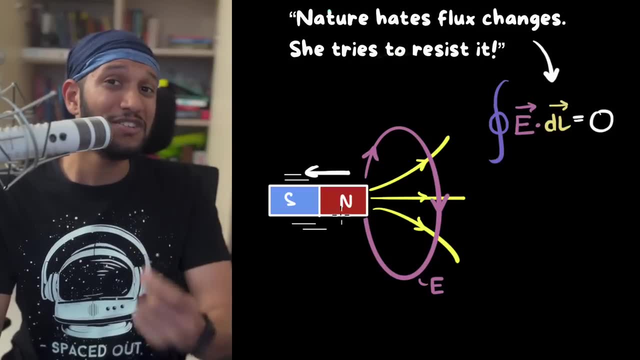 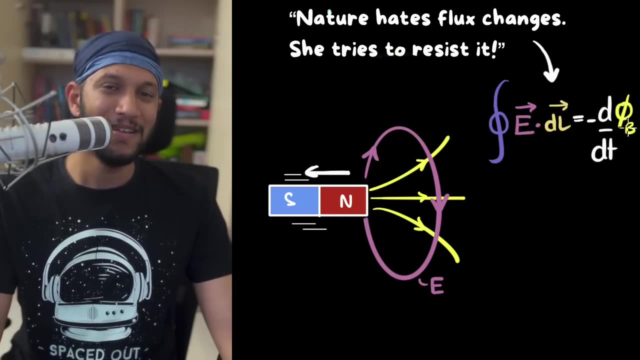 is it We just saw from Faraday's experiment. This is the work done. This is the energy that the electric field is transferring and that equals how quickly the flux changes. Mathematically we write it as d phi over dt: The rate of change of flux. 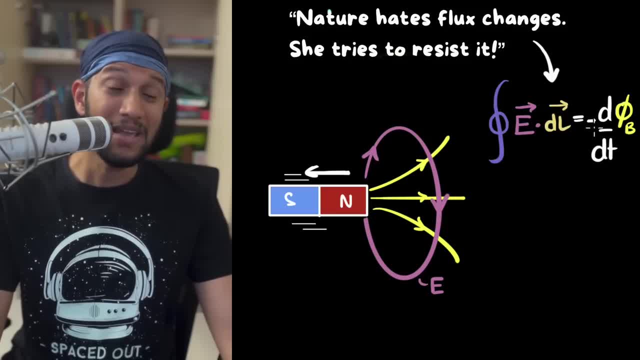 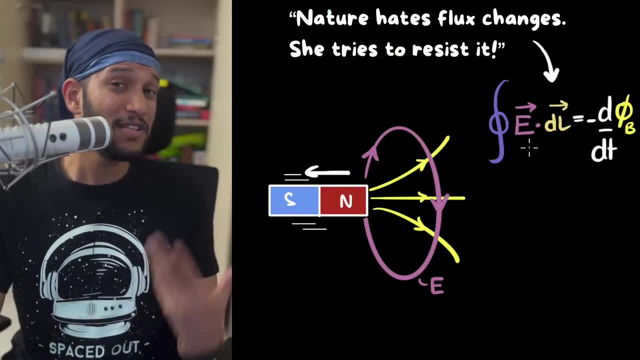 And why is there a minus sign, Feynman? Well, the minus sign is basically this point: that she tries to oppose it. If the flux increases, she'll put an electric field in such a way as to try and decrease it. And if the flux decreases, 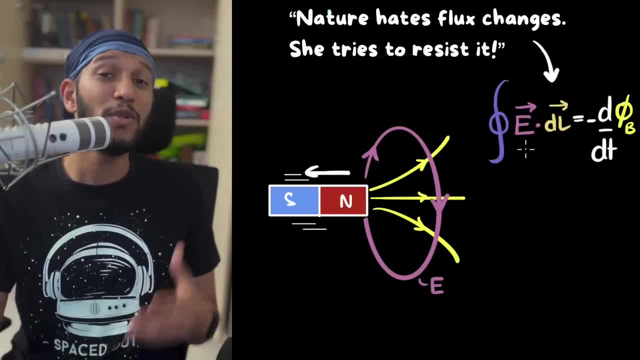 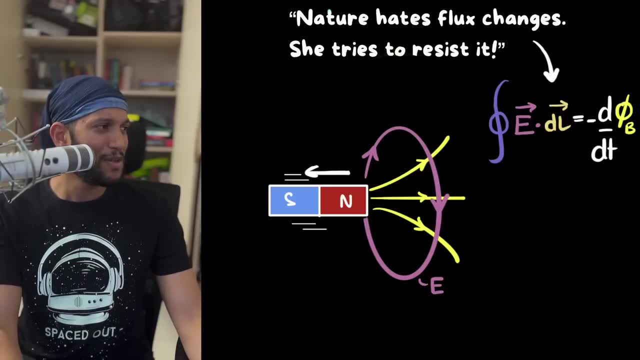 she'll put an electric field in such a way as to try and increase it. Nature will always try to oppose the change in flux, And that's what this equation is saying. But I'm a little confused, Feynman, Because earlier we said it's zero. 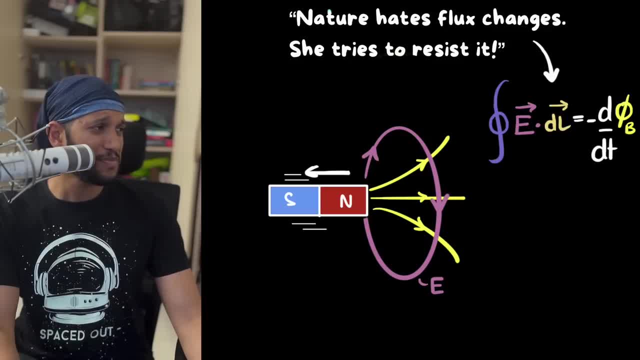 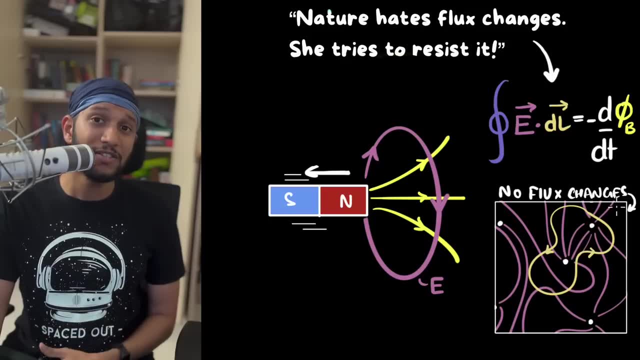 Now we're saying it's not zero, Like what does it all mean? Like how do we put it all together? Well, it says: well, if we are. earlier we were dealing with electric fields, static electric fields, where there were no flux changes, If there. 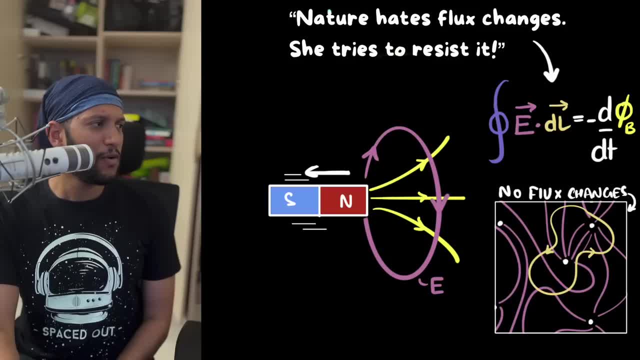 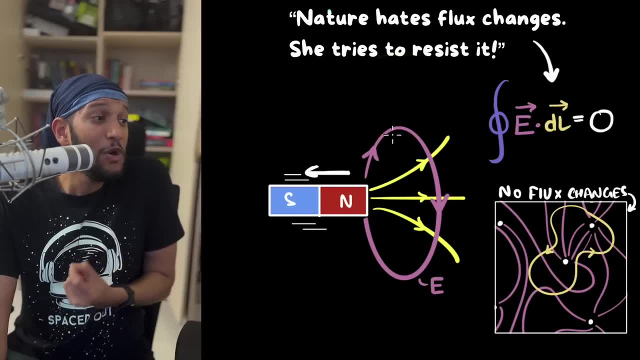 are no flux changes, nature has no problem. And now we go back to our original. the work done in a closed loop would become zero. But now, whenever there is a flux change, we have a new kind of electric field. Look, this is no longer a radially symmetric. 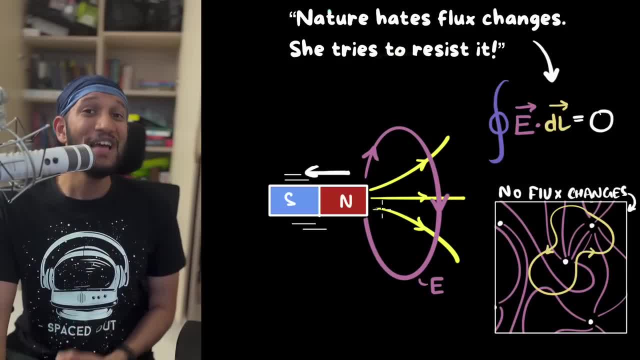 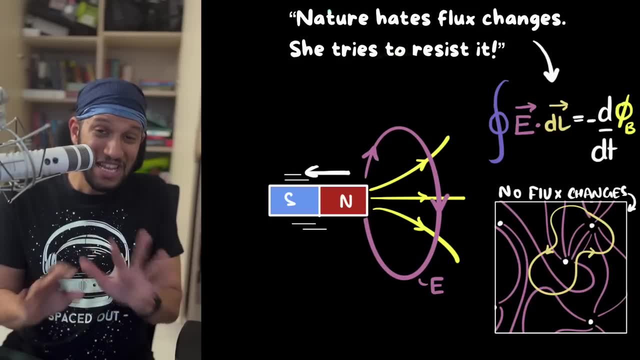 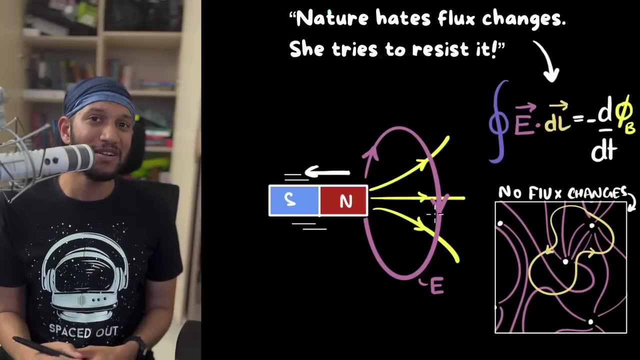 electric field. When you have this field you do have work done in a closed path now and that work done becomes minus d phi over dt. So in general, if you have both radial fields and these induced looping fields created by changing magnetic flux, in general the work done in a closed path won't be zero. 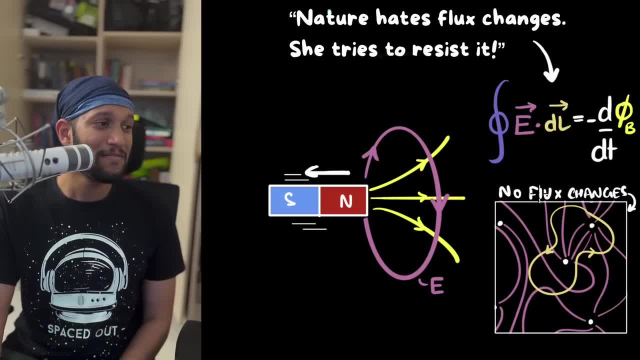 It will be negative d phi by dt, But in most of the circuits that we are dealing with, the flux changes are not there, And that's the reason why, in most cases, we equate this to zero. That's the whole story. Lastly, you said this is how our world.